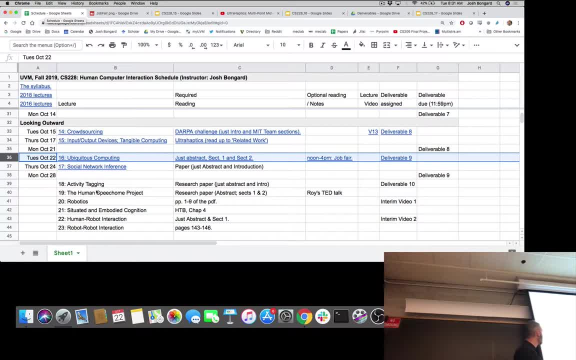 we're going to finish the last couple of slides in lecture 15, which is sort of broadening our discussion about interactive technology, where we're looking now not at GUIs or graphical user interfaces but thinking about how to bring into account the other sense organs like audition and 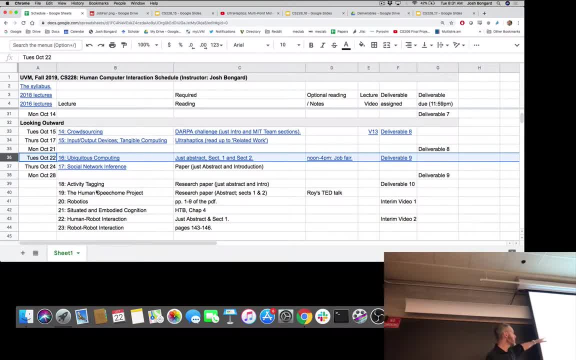 touch, And we'll finish our discussion of touch today. We'll talk a little bit about the other sense organs like audition and touch. We'll talk a little bit about what ubiquitous computing actually is. We will finish this lecture today and start in on the first of three lectures we're going to have that look at. 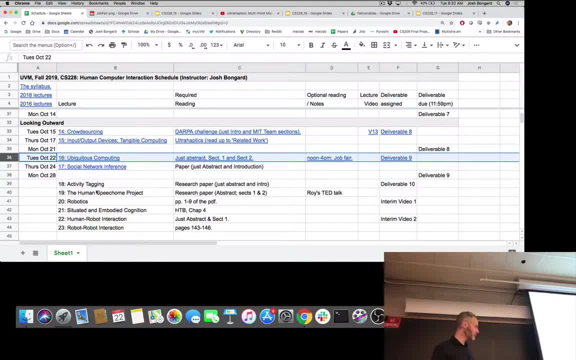 deploying a particular kind of ubiquitous technology to ask and try to answer a scientific question that would be difficult or impossible to do without technology which is threaded into the physical environment. Okay, so that's where we were and where we're going. I'm going to 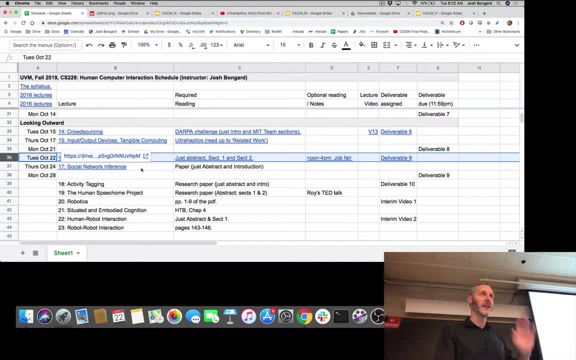 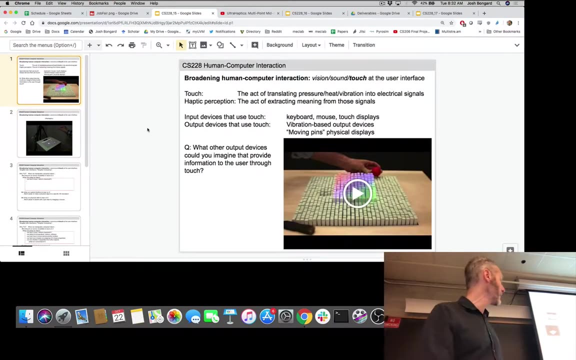 start lecture and then we're going to come back to Deliverable 9 about partway through the lecture, because I want to introduce the concept of scaffolding, which is what you're going to be tackling in Deliverable 9.. Okay, so, just as a reminder, we ended last time by talking about 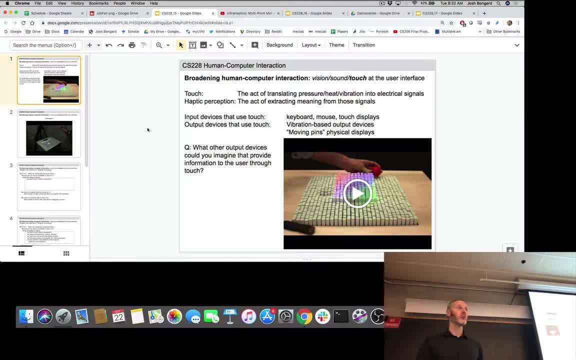 tactile user interfaces. Can we create technologies that communicate back through us through touch, And what would be the advantages of communicating through touch rather than projecting a visual feedback? What were some of the advantages we talked about last week? We talked about TUIs. Why bother creating a moving pin display that we can actually feel? 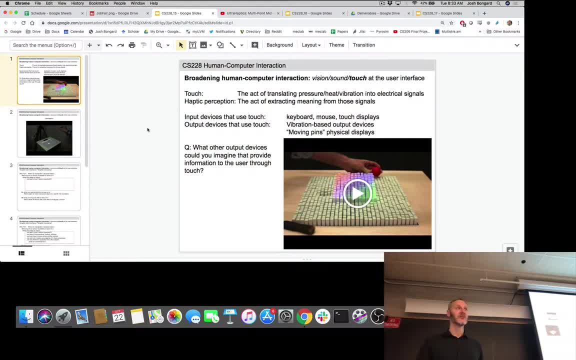 feedback, physical feedback from the device. You can actually physically interact with that space that's away from you, Absolutely right. So this idea of physical interaction: if we're interacting with someone or something else, a lot of that communication is through touch and through. 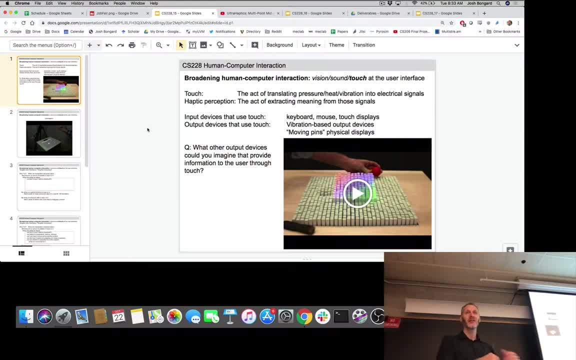 skin right. We can imagine through tactile user interfaces that multiple people and multiple computers or technologies can collectively manipulate objects and create or do something together. And there is an important aspect of tactile feedback in that process. I skipped over last time ultra haptics, which I think is a particularly 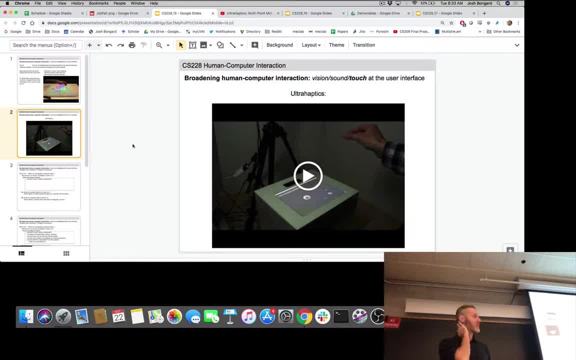 interesting example of a tangible user interface. This one is going to, as you'll see in a moment, provide tactile feedback, but also visual feedback, and combine them in an interesting way. So let's have a look at ultra haptics and then we will talk about the technology itself. This one: 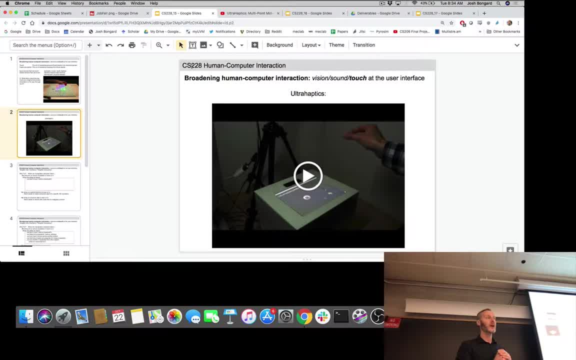 pay particular attention to the feedback loop. We talked at the beginning of the course about the output, or the interaction of the user becomes the input to the device and vice versa. That feedback loop exists here, but it's a little bit difficult and a little bit subtle to see what is involved in that feedback loop. Okay, let's have a look. 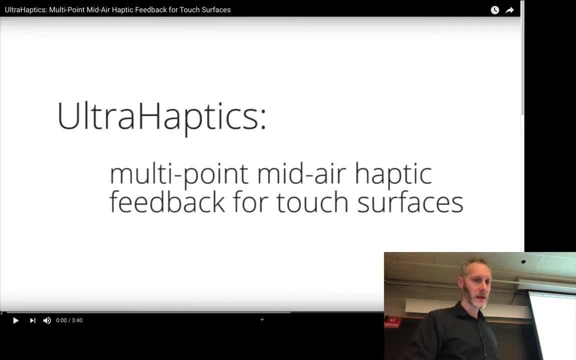 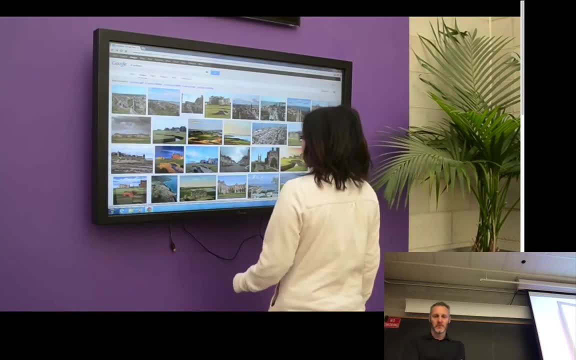 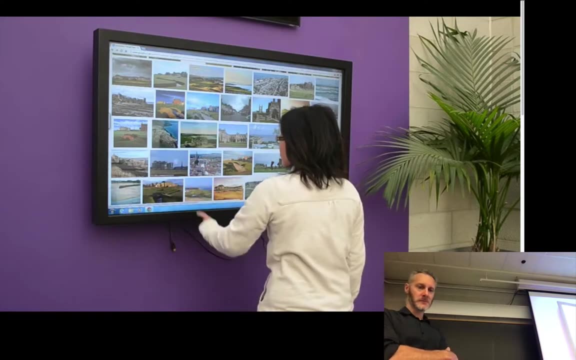 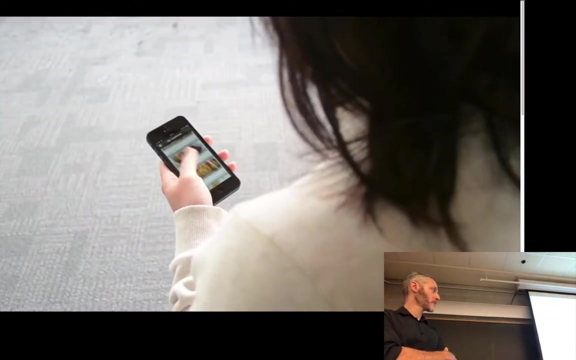 Interactive surfaces are now common in every. Interactive surfaces are now common in every day life. They allow users to walk up and use them with no instruction. Second, current methods for providing tactile feedback require the user to cover up the visual content by touching the display or attach devices. 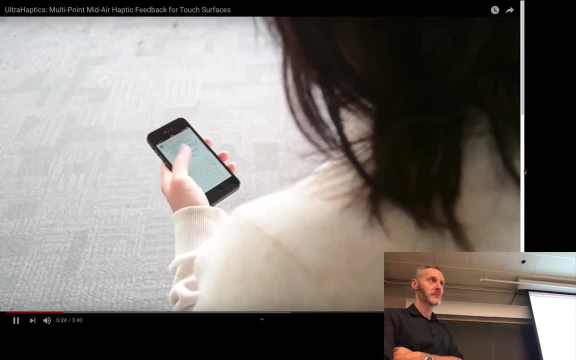 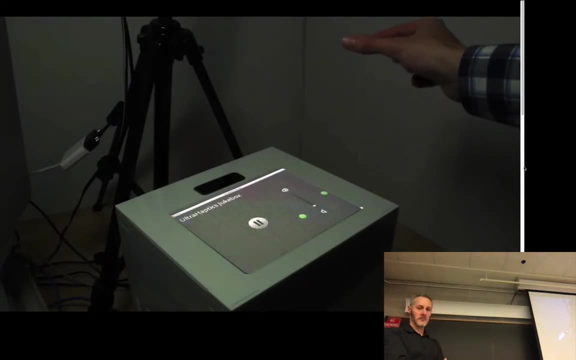 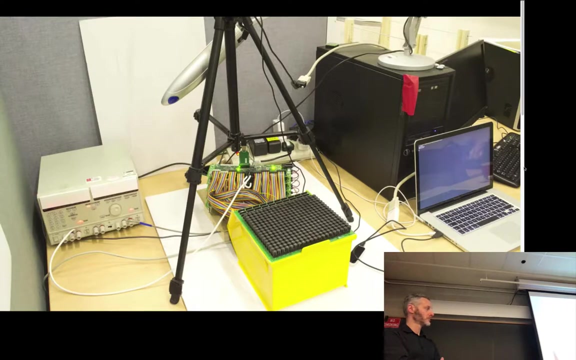 to their hands, For example for the search engine. in the factory. we present Ultra haptics, a system that provides midair haptic feedback and requires no contact with either tools, attachments or or the surface itself. UltraHaptics uses a phased array of ultrasound transducers. 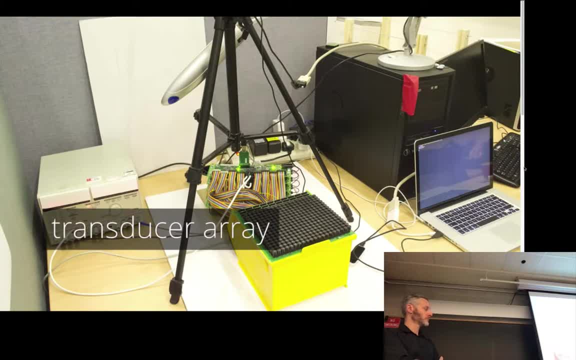 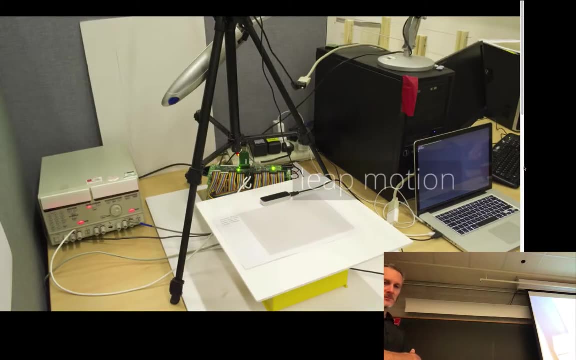 to create tactile focal points in mid-air. The array is driven by a stack of five driver boards which receive emission patterns from a PC. The user's hands are tracked by a leap motion controller and the haptic feedback is projected through an acoustically transparent display. 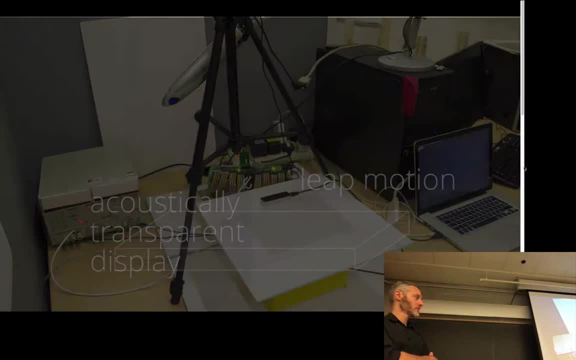 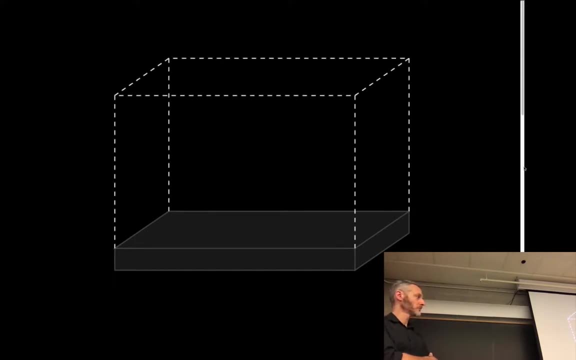 directly onto the user's bare hands. There are four steps to our unique focusing method. First, we define a large volume around the transducer array within which we will model the ultrasound field. Then we position positive control points where we want to form focal points. 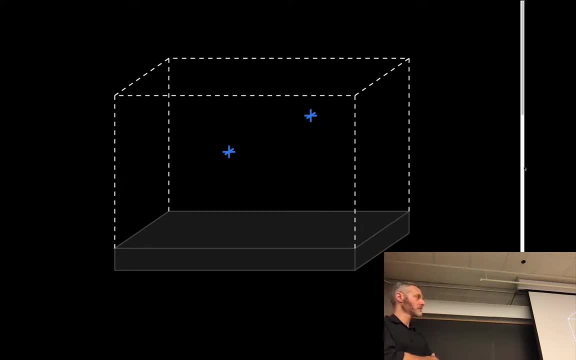 These tell the system to generate the highest intensity ultrasound possible at these locations. They are then surrounded with null control points. These have the opposite effect, telling the system to generate the lowest intensity ultrasound at these locations. Finally, the phase delay and amplitude are calculated for each transducer in the array. 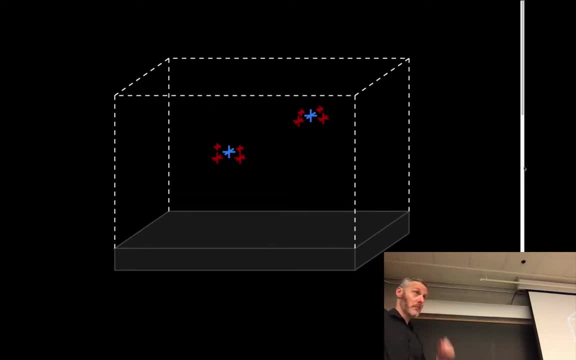 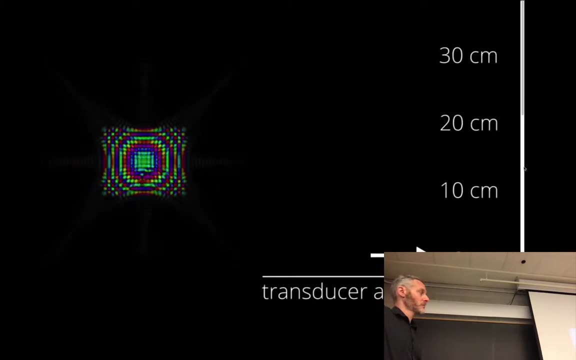 to create an acoustic field that matches the control points. This simulation illustrates the acoustic field as we move up from the transducer array. Color represents phase and brightness represents intensity. At a height of 20 centimeters, a focal point is formed. 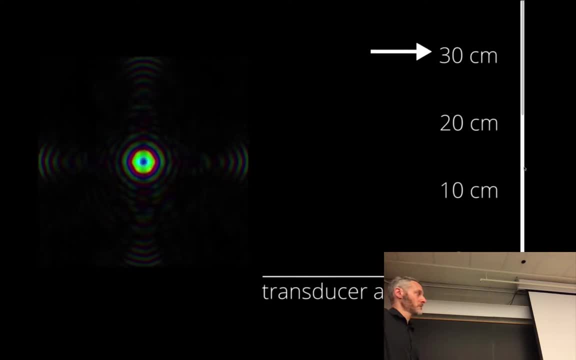 Above the ultrasound defocuses once more. Similarly, this simulation shows five discrete focal points being formed at the same time. By varying the tactile properties of focal points, such as the frequency, they can be made to feel different from each other. 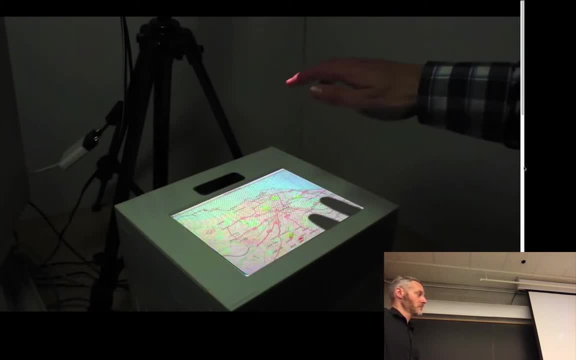 In this scenario, a tactile information layer is created above the display. By moving their hand over the map, the user can feel the population density of a city. The frequency, which is the density of the population density of a city is the density of the transducer. 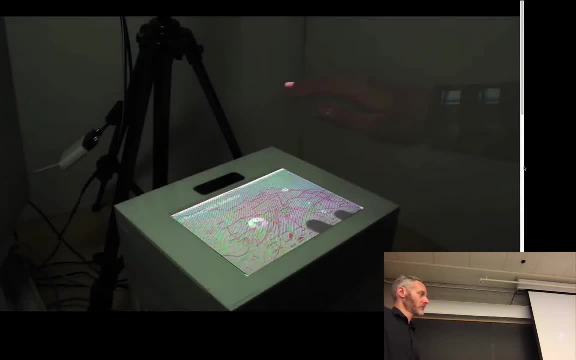 The frequency, which is the density of the population. density of a city is the density of the transducer. The density of a focal point represents the density in that area. Here focal points are created above elements of a music player interface. This allows a user to locate themselves on the interface without looking. 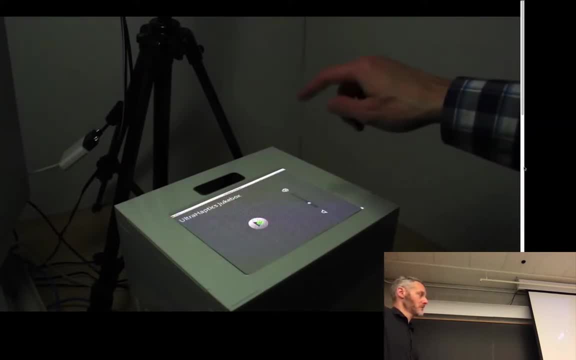 Tapping the focal point above the button starts and stops the music. The focal point above the volume slider can be grabbed. At this point it pulses to inform the user that the music is being played. The system has recognized their grasp. The focal point can then be slid up and down to change the volume. 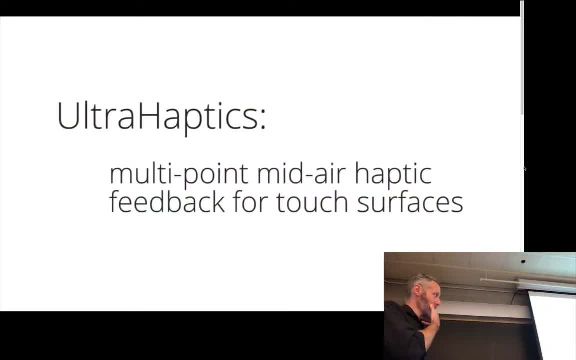 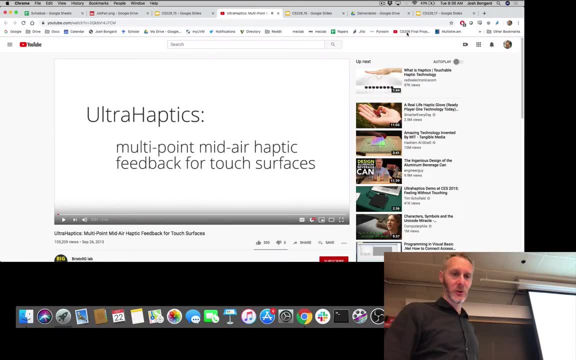 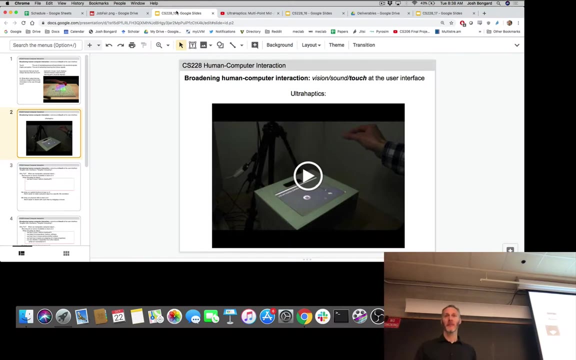 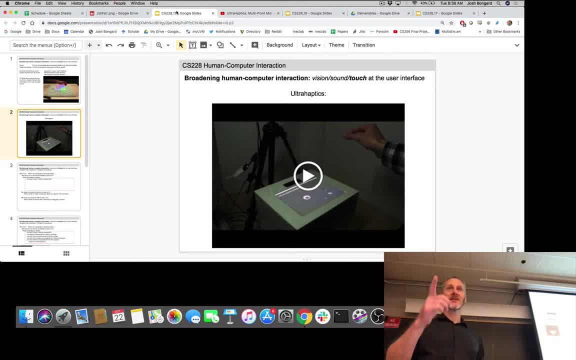 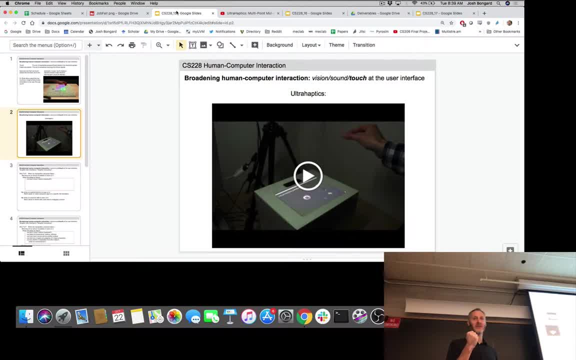 That's the input to the UltraHaptic system. What is the input to the user? Well, it's the screen. So yeah, and I apologize for the sound, You can go back and watch the video at your leisure. So these phased arrays that are underneath the hand or, in some cases, in this case, projecting from above downward, are a set of phased ultrasonic emitters. 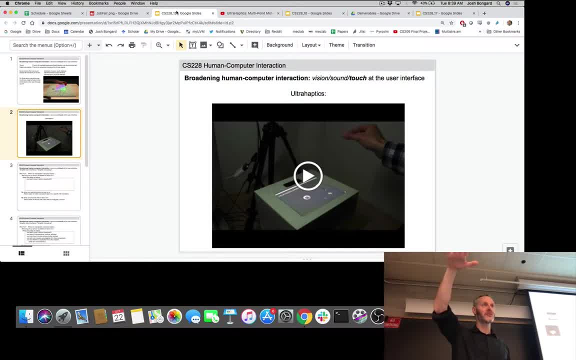 So they're emitting ultrasound, which is not unlike the infrared in the Leap Motion Device. It's a physical phenomenon that sends out a wave and, in some cases, detects the sound, So you can see the feedback from the wave, But in this case the wave that's being emitted is felt by the user's hand. 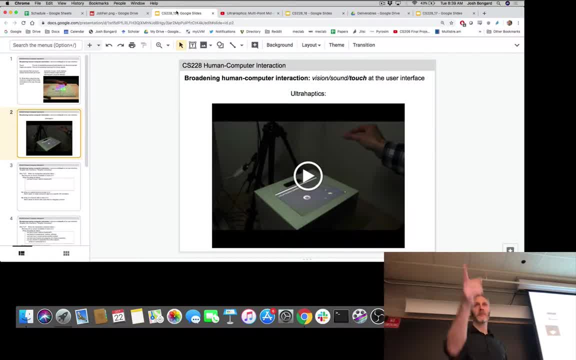 How In point locations they can draw that Absolutely. They mention these positive and negative focal points. So these phased arrays are all emitting a series of ultrasonic waves And the device itself can control the wave. It can control the phase offset of the waves and the frequency of the waves. 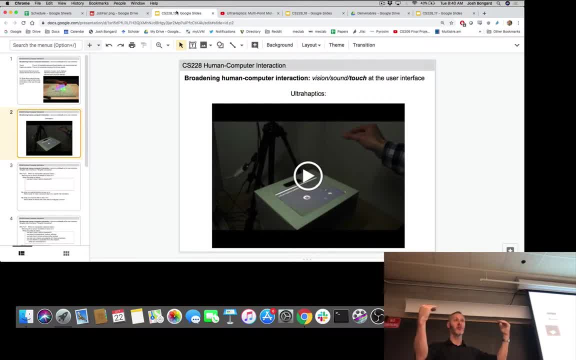 So you've all probably seen a body of water. You have two waves that are approaching one another And if they hit in just the right phase, if they come together at the same time, they produce positive interference. You get a wave that is larger than either individual wave. 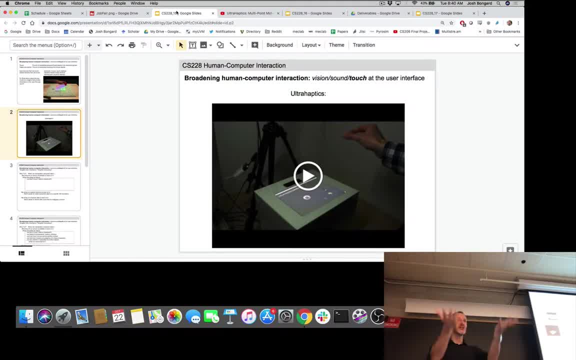 That's, in this case, the positive focal point. Imagine these waves that are coming out of the bottom of the phased array. If the phased array is placed above the hand pointing down, these waves are coming down And these waves are hitting one another at an exact position in three-dimensional space. 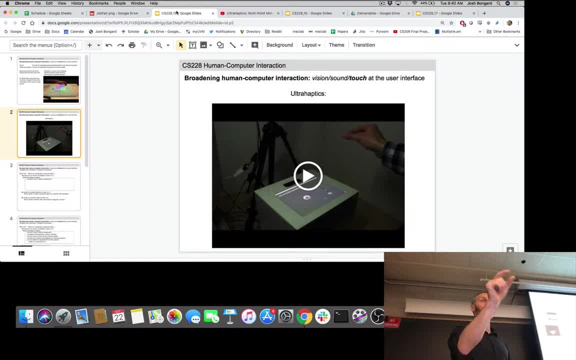 And if your fingers happen to be very near that positive point of positive interference, you feel a vibration which feels something like something is there that is resisting your grasp, And you can see in this example of the music player interface. you could simulate something like this. 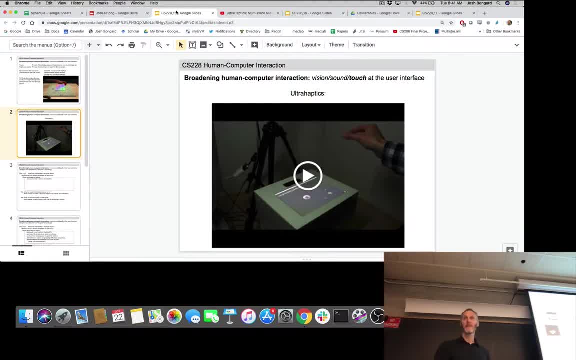 You could simulate something like a knob or a button or a key press. I have a question. I mean so it sounds like they're kind of sound waves or whatever. They're sound waves absolutely at a certain frequency. Does it make any noise to the human hearing? 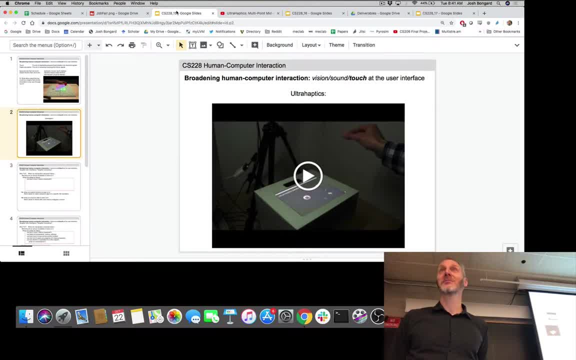 No, it is beyond human hearing, which is kind of interesting. You could imagine also adding in an auditory feedback: You can feel these waves rather than hear them. Okay, so that's a positive interference point. You can create a negative control point where you set the phase offset so that they are out of phase. 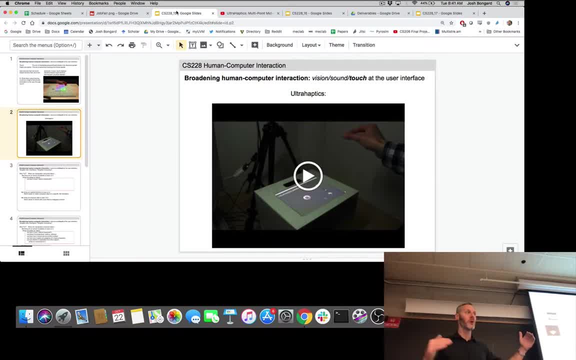 And again you've seen in a body of water two waves that approach one another and they're off by a little bit and they sort of cancel each other out and you get mean height right. So in this case they create, if they're trying to simulate, a knob that can be grasped. 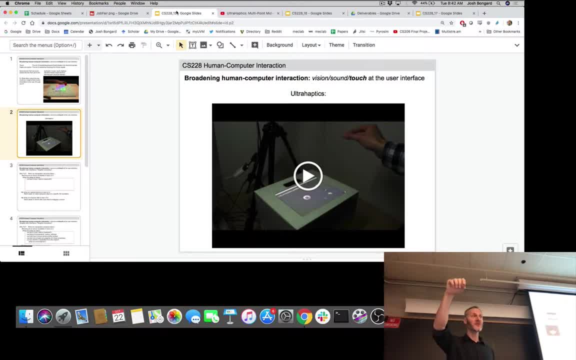 they project or they set the frequency and phase offsets of these ultrasonic emitters to produce vibration at this point. So you can see that they're at this particular point and everywhere around that point they're trying to cancel out these waves, minimize their frequency. 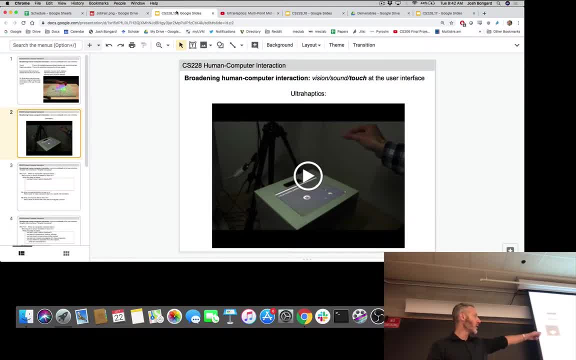 so it doesn't feel like there's anything there, right, That's creating a discrete point in space. And then they gave this sort of example of a map where you have some continuous increase in interference, which feels like something that's increasingly rough. 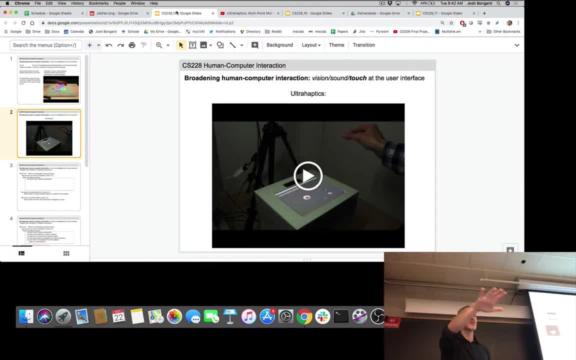 Obviously there's nothing there, But it gives the perception that when you move your hand over the map you're feeling increasing population density or some distribution of data distributed over a two-dimensional plane. That's the idea Kind of interesting and neat, but why would one want to do that? 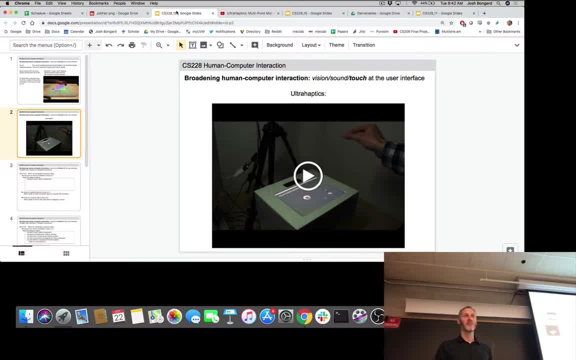 What's the advantage of being able to simulate a three-dimensional object that someone can reach in and manipulate, even when it's not there? They showed you a couple applications. How else might this be useful? Well, maybe if you've got a behind-the-view or a visual impairment. 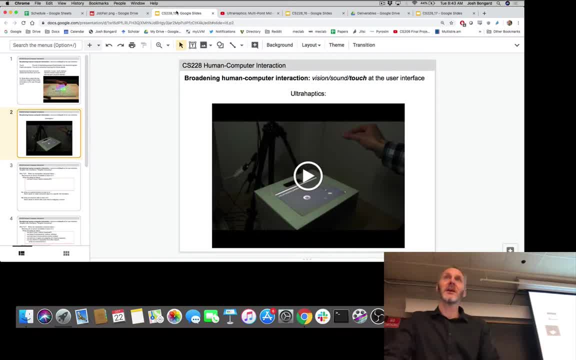 Absolutely right. So there's a visual component to this particular application, but you don't necessarily need a visual component. Other ideas: They mentioned in passing in the video that this might be useful for applications where the user doesn't actually need to be looking where they're grasping. 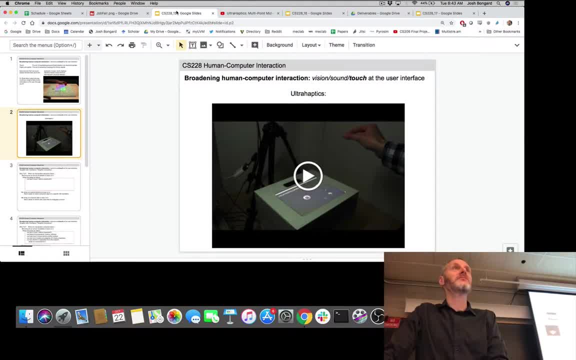 Maybe in outer space an astronaut you know could love their early days. that could be useful in that context. Absolutely, it could be useful in a case like that. There are a lot of domains where they pay very careful attention to heads-up display. 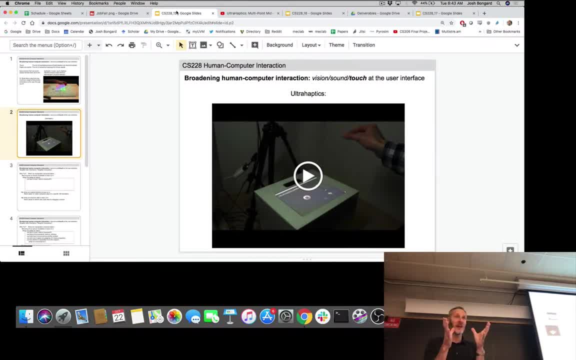 like working on the space station or other off-Earth applications. In military applications, there's a lot of potential information and you need to think very carefully about providing enough information for the human user to make intelligent decisions in real-time, but obviously not overwhelm them. 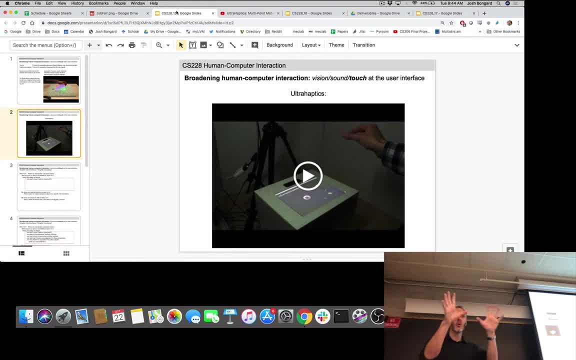 One strategy is not to simply produce more and more visual feedback, but to take feedback and shunt it to different sense organs. So there's visual display and tactile display. If I'm focusing on something visual, I might be able to reach outside of my visual field. 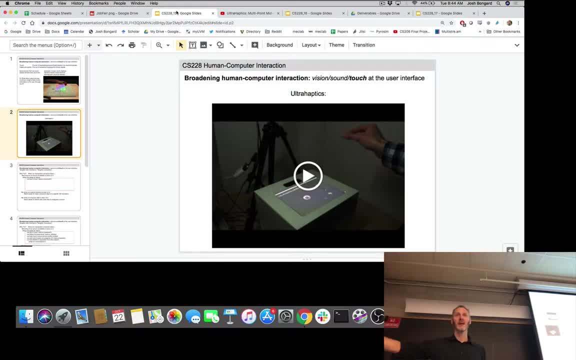 and feel something and manipulate it without having to take my attention off whatever it is that I'm looking at. You could have this in a public space where sanitary concerns could be something a lot of people are handling a touch screen and whatnot. 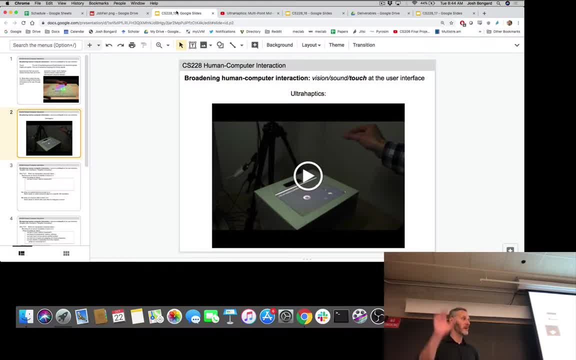 Yeah, absolutely. That's a great example, right? A social context where you prefer people aren't actually touching an object, Or you maybe can develop a game. then you can play the game by their head. Absolutely right. It'd be kind of interesting to be where you're reaching in and manipulating arbitrary objects. 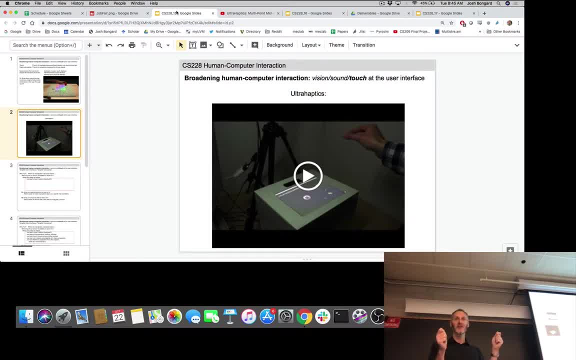 Imagine that you have control over the frequency, the frequencies and phase offsets of this array. How complex an object could you project that would project the illusion of that object actually being there? Imagine trying to do that and ask your user to reach into this field and describe the. 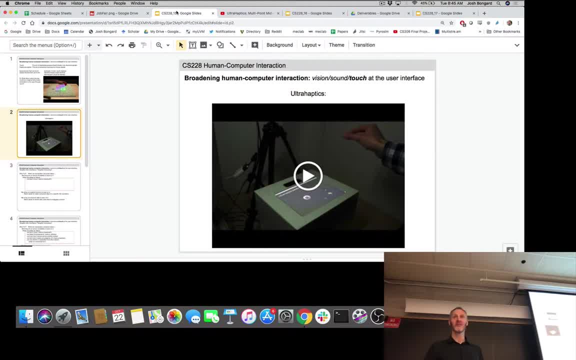 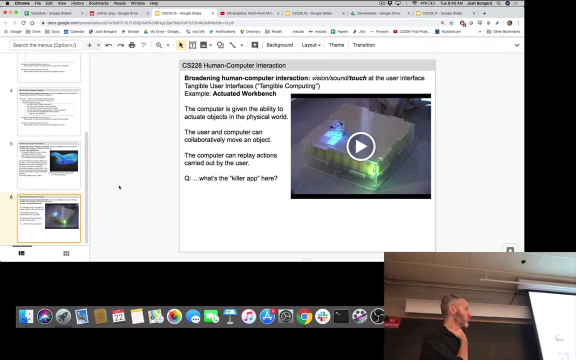 object that's inside the field of the array Could be kind of interesting. Imagine a lot of potential applications. Okay, So I introduced last time but we didn't have a time, a chance, to look at it. The second application. this is the actuated workbench. 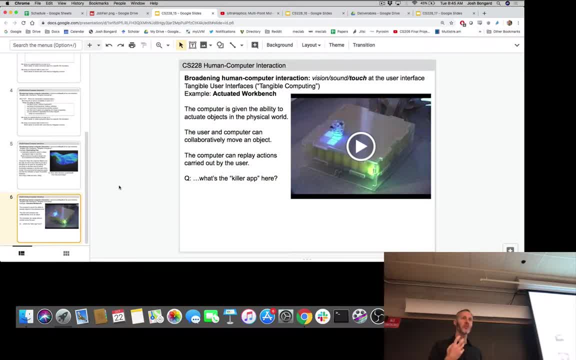 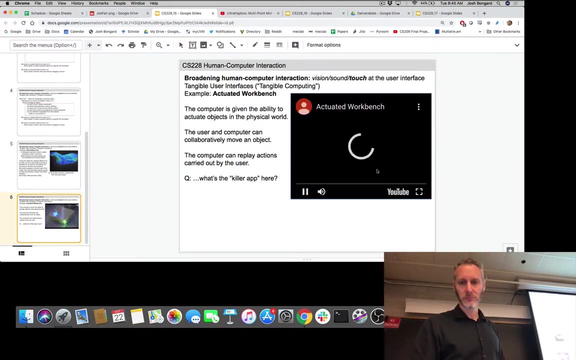 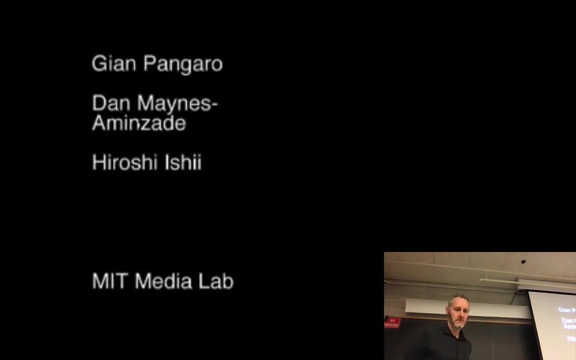 If we can create a feedback loop where the device is also providing physical feedback to the user, you can imagine users and the technology itself collaboratively manipulating, in this case, a real object. The actuated workbench consists of an eight by eight array of electromagnets. 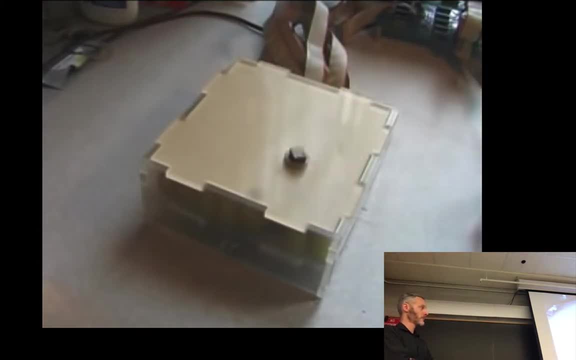 It uses magnetic attraction and repulsion to move magnetic objects two-dimensionally on a flat surface. Here we can see a magnet moving in stepwise Manhattan motion. Here we see an object moving in a smooth circular pattern, Although the array of electromagnets is fixed. 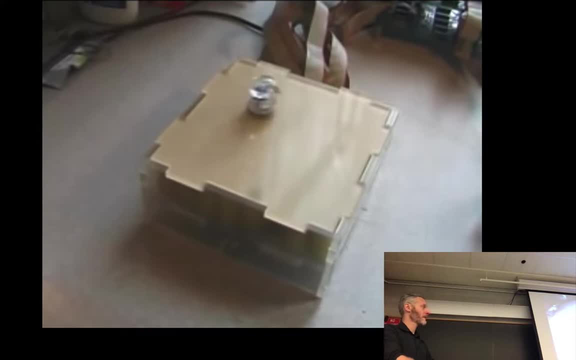 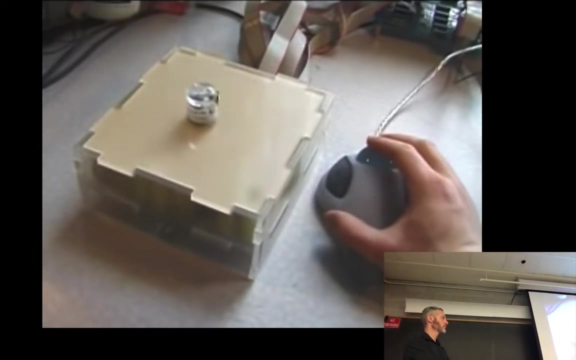 the system can create smooth motion by varying the strength of the electromagnetic fields. Okay, In addition to magnets, the electromagnetic array can move any small ferromagnetic object, such as a paperclip. Here the user controls the puck's motion with a trackball. 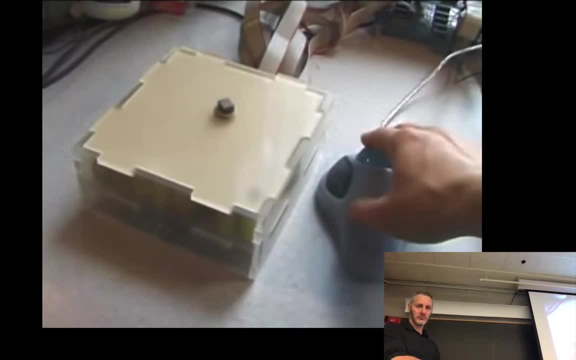 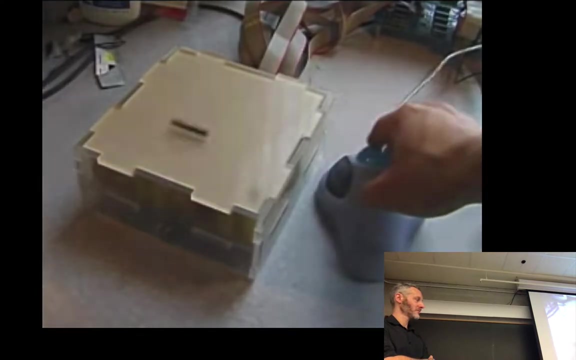 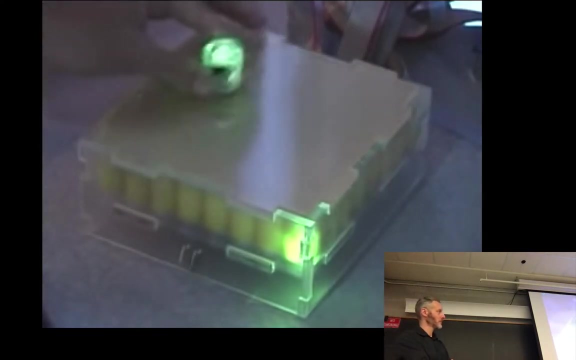 Okay. Smaller objects can move much faster, though their motion is not always so smooth. Magnets of different sizes and shapes behave differently in the system's magnetic fields. This stack of small magnets comes around musically. We use computer vision as a preliminary object tracking technology. 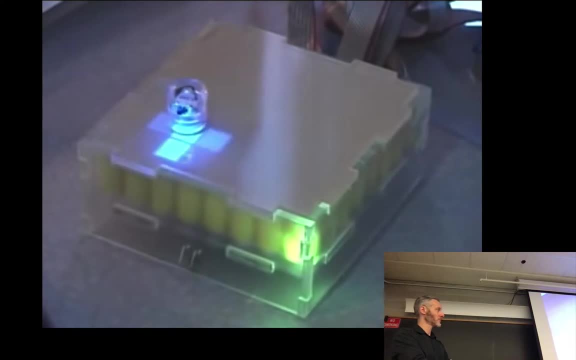 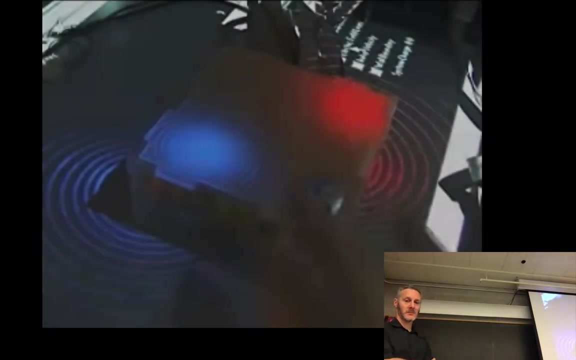 Here the user records a path by moving the puck on the surface and the system then replays that path through magnetic actuation. The blue projection around the puck is a graphical visualization of the strength of each adjacent magnetic field. Here is an example application intended to teach users about physics. 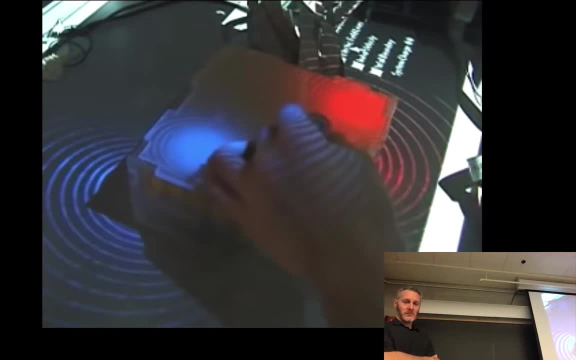 The red projected area on the surface represents a zone of attractive force, while the blue area represents repulsive force. The user can feel these forces by lightly holding the puck in different areas of the board. When the user releases the puck, it flies to the red zone of the board to which it is. 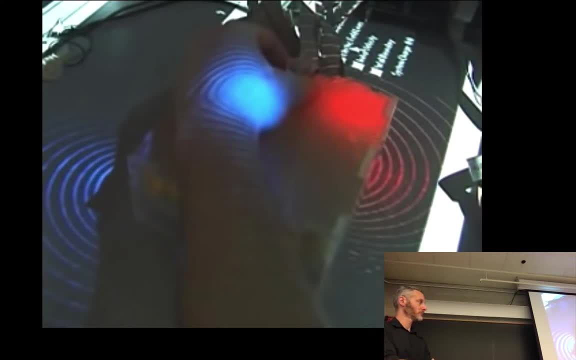 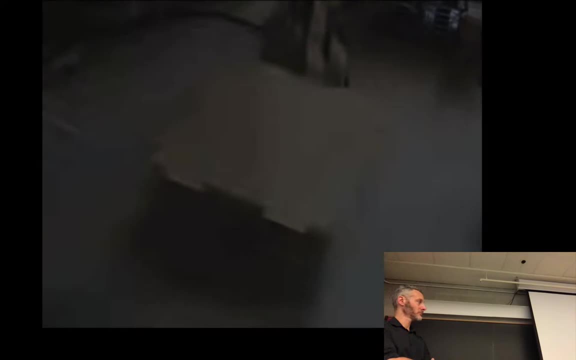 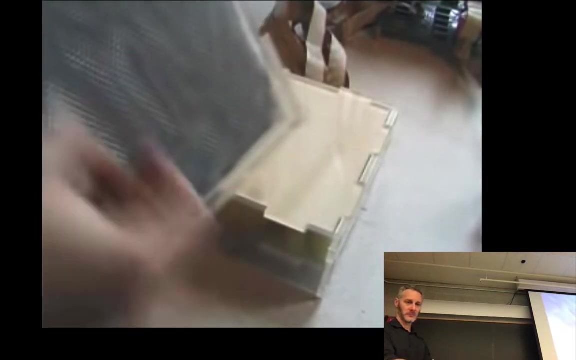 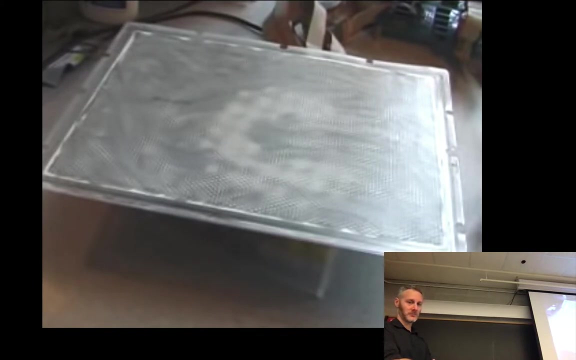 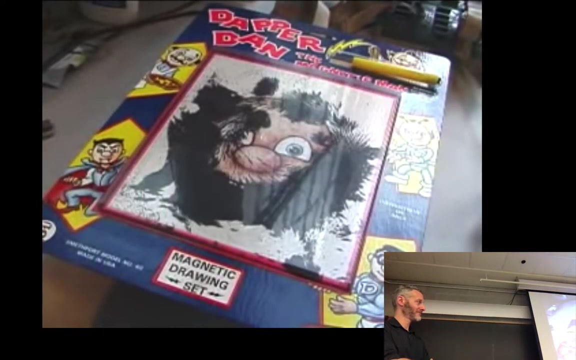 attracted. Magnetic drawing toys are effective for visualizing the actuated workbench's magnetic fields. A magnet doodle allows us to see the fields used to trace the smooth circular path shown at the beginning of this video. The dapper Dan toy lets us see the magnetic activity in the movements of iron filings. 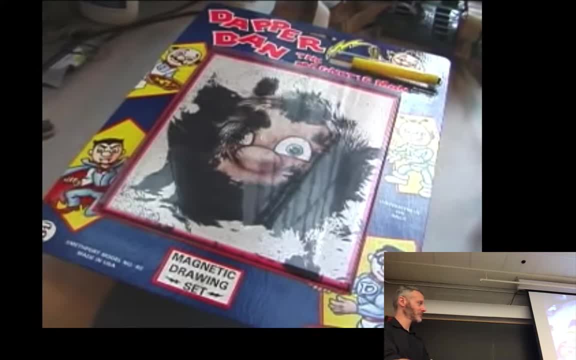 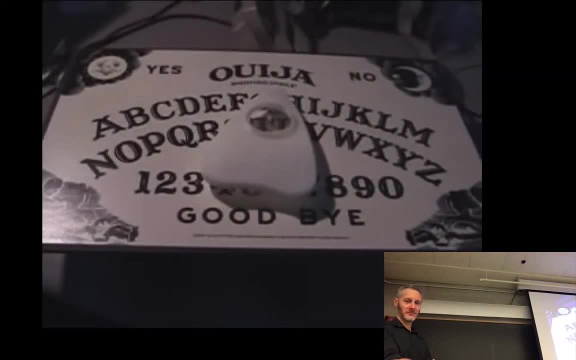 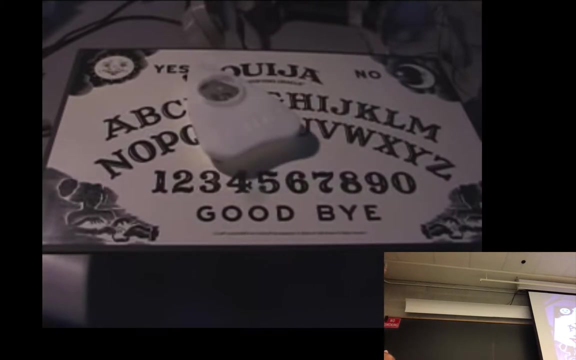 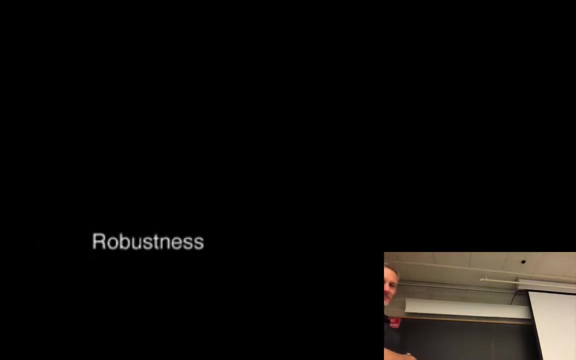 on the surface. The actuated workbench can be used to control man-made grabbing patterns, Women's burping animations. 하루 control the planchette in a Ouija board game. very practical like other robust systems such as the diamond touch presented by Mitsubishi. 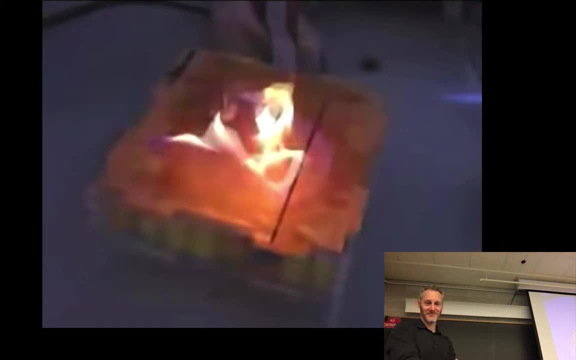 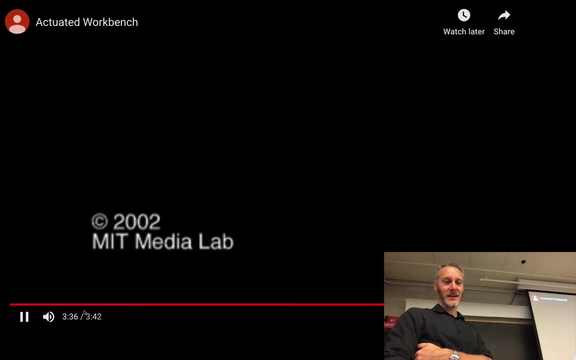 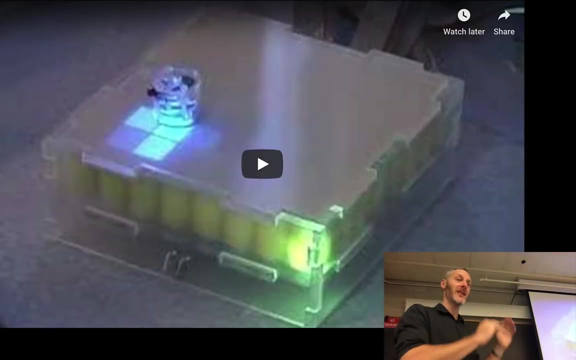 electric research labs in WIS 2001. the actuated workbench works even when set on fire- the last very important demo there. of course, that's a nod to robotics demos. whenever you create a video of your robot, you should always set it on fire at the end to demonstrate it's very robust. okay, actuated workbench, what's? 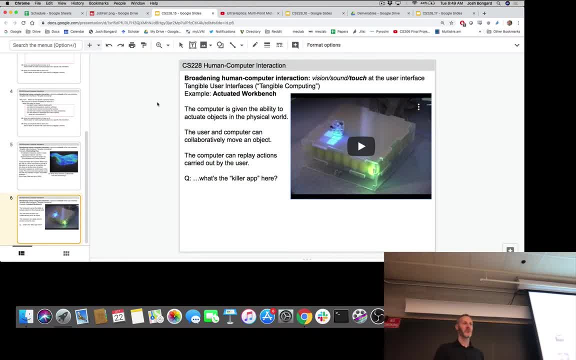 the feedback loop here. so we just saw ultra haptics where they're using ultrasound to create this tactile feedback loop. what's the physical phenomenon being exploited here? electromagnetic waves or fields, right, okay, so what does this feedback loop afford? we saw a few examples of feedback between human users. 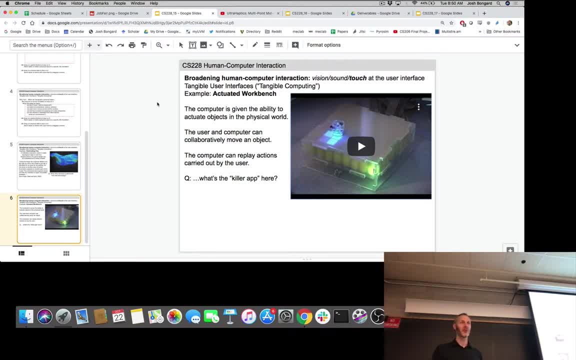 and the device. what are some of those collaborative actions that the two can perform using this technology? okay, so what you see here is an experience that's developed by GPS here, and this is the pretty easy to use. interesting thing is that a coin that we use to generate solar energy is a really good way of generatingrons. that 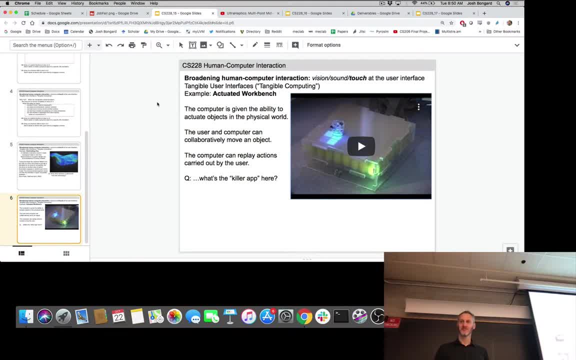 are not going to generate energy, they're just going to have to do is, and, I think, fields, which is why Juno, their spacecraft, has to be large enough so that it can get sucked into the field of Jupiter and raise billions of tax money. 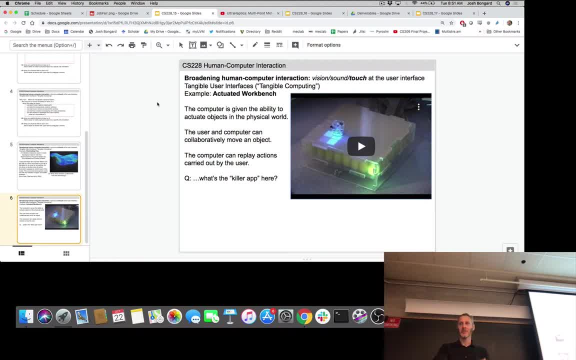 So having something like that would be great to simulate the field of a planet or the sun, to see how, over time, it could interact with spaceships or planets nearby, Sure, right. So an educational or training application. you can imagine a lot of educational applications. 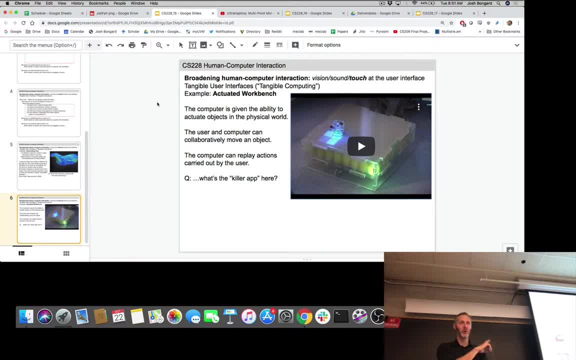 here. How might these applications? if you were to create an educational application or a training application with this device, what advantages would it have over a more traditional way of teaching electromagnetic fields and interactions of large bodies with electromagnetic fields- Moving objects in real time right? 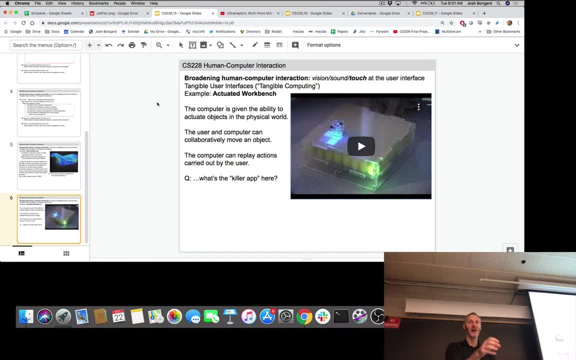 You can see the object itself And if you hold on to the object, You can physically feel the effects of an electromagnetic field which we can't see on objects. One of the biggest challenges in education is taking an abstract concept and trying to make it concrete in some way, right? 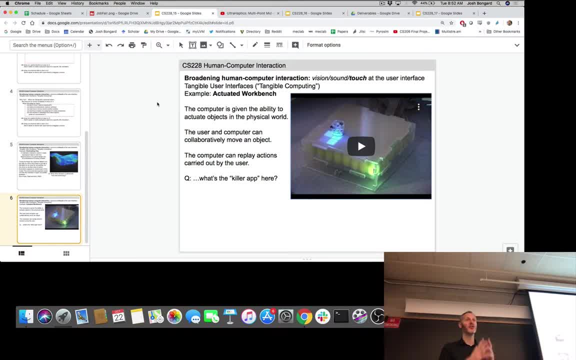 So you can imagine the actuated workbench here as providing unique opportunities to concretize particular abstract concepts like electromagnetism. Okay, Forget electromagnets for a moment. What else might you be able to teach better using this technology than others? 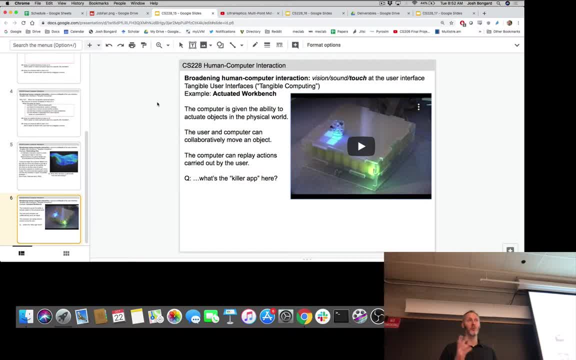 You are all in the process of building an educational system and hopefully the Leap Motion device will provide you and your users with opportunities to learn ASL better than if you just showed them a whole bunch of YouTube videos and they practiced in response to the videos. 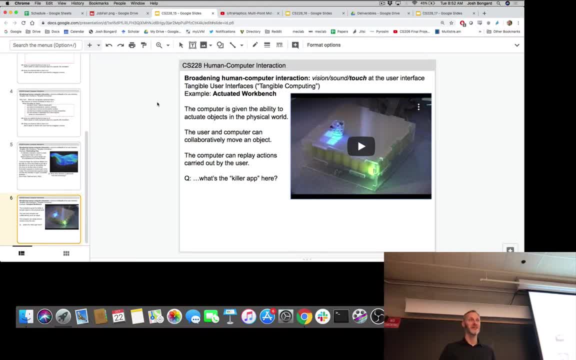 There's something about the interaction with the Leap Motion device that facilitates learning and what here might be able to facilitate learning over doing it in a more traditional sense. I like the process of motion, so things like algorithms, like if there's a lantern, it's. 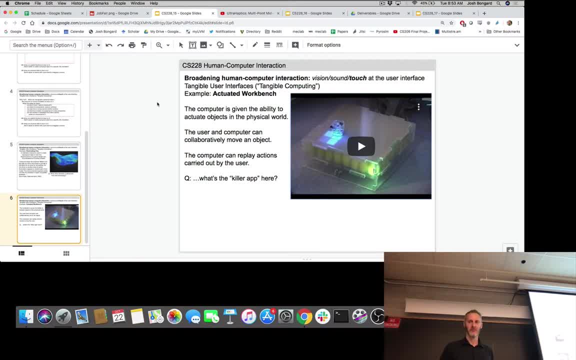 ants. so that type of algorithm: you go left and go right and you could physically see if you had someone program a robot or perform an algorithm, the course it would go Okay. So you could program Chris Langton's ant, which is a simple agent, and learn a little bit about AI and path planning. 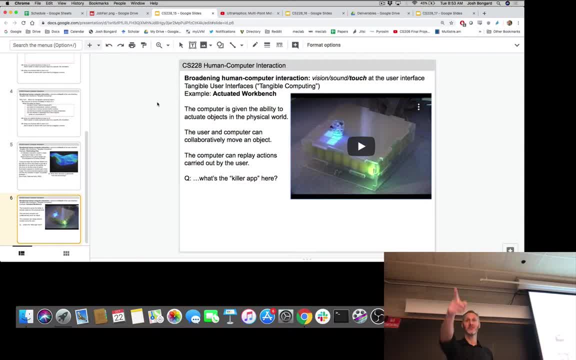 What other domains might it be useful to teach using this device? Chess, There's an interesting idea. Yep, How many of you have learned to try and write in another language? I've learned Kanji or some other language. that requires fine motor skills. 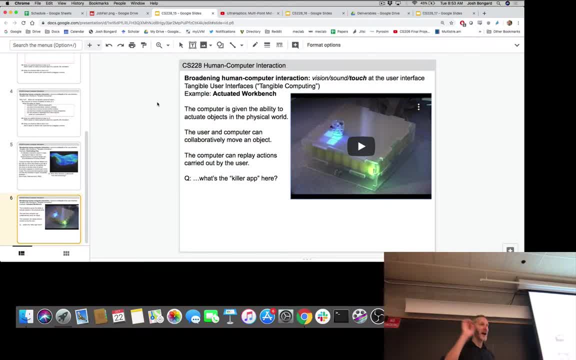 Imagine someone, an expert in Kanji, signing They're going to draw various symbols using this device and then the user holds the device and their hand is pulled through the process of drawing Kanji characters. You could imagine for teaching languages or written expression. perhaps that would be. 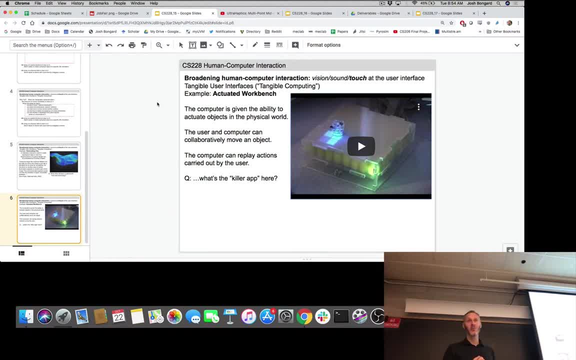 useful. One of the biggest challenges in learning a sport or chess or anything that's tactile- writing a language. obviously it has a lot to do with the hands. You can watch the hands of the teacher From a distance and try and replicate that with your own hands. 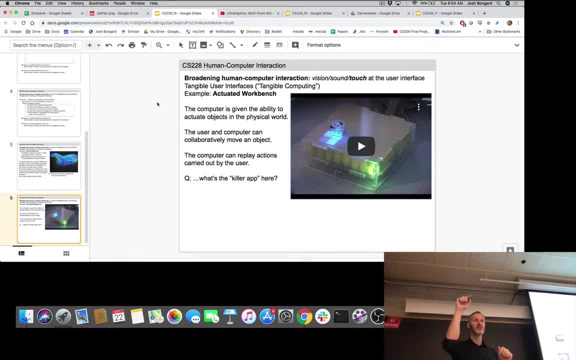 Very difficult to do, because you're going from the tactile sense to the visual sense and translating back into your own tactile sense. It would be nice to cut out the middleman vision in this case and allow, in a sense, the teacher's hands to become your own hands. 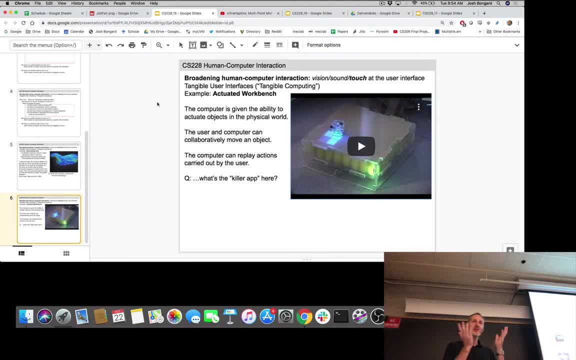 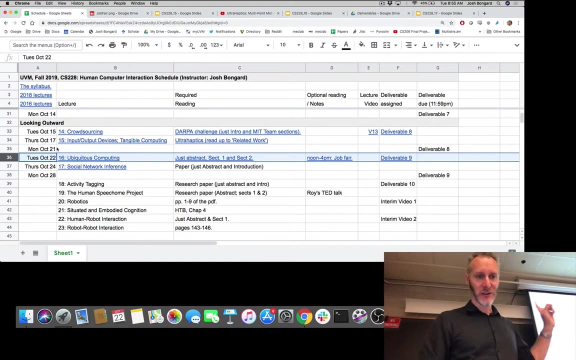 You could imagine whether that would work or not, but that's the way of trying to think about this. right, We want to try and come up with unique learning opportunities That would be difficult or impossible to do without the technology itself. That concludes our discussion of tactile interfaces. 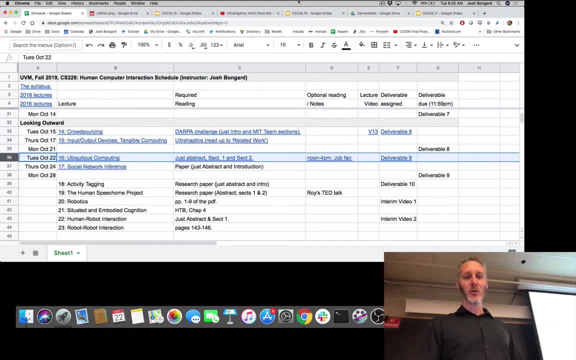 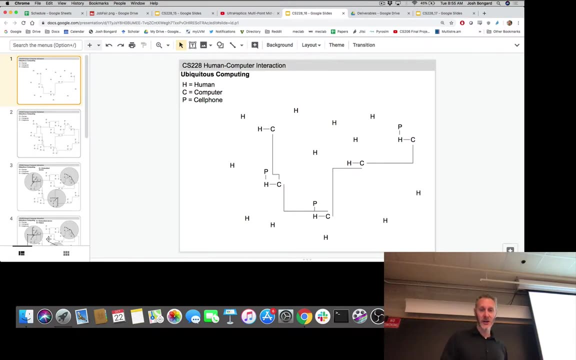 We're going to switch now and talk about this general field of ubiquitous computing, which is a subfield of HCI. We're going to stitch technology directly into the physical world, and what are some of the unique challenges there? I started the beginning of the semester with this little cartoon here. 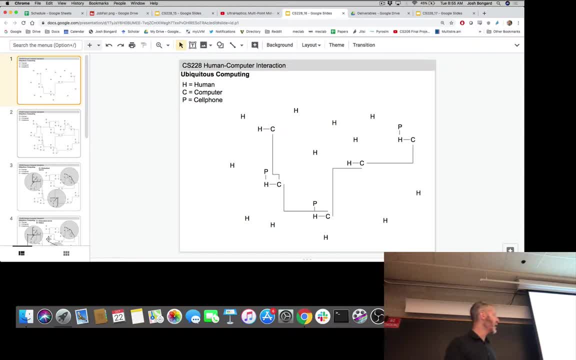 Um the stone age we had all these humans and a small minority of them had desktop computers, and within a few years there were more many more cell phones out there than laptops and desktops. cell phones and traditional computers have lots of differences, but for our purposes, our phones are interacting. 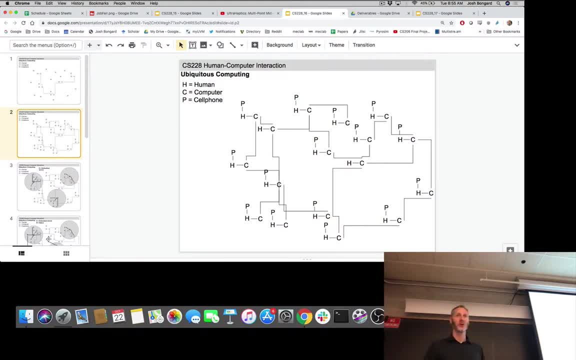 with us, but also interacting more directly with the real world than our computers are. modern smartphones have a large number of sensors in them which, unless you turn them off, they are recording various information in real time. we're going to start in the applications, uh, in the next. 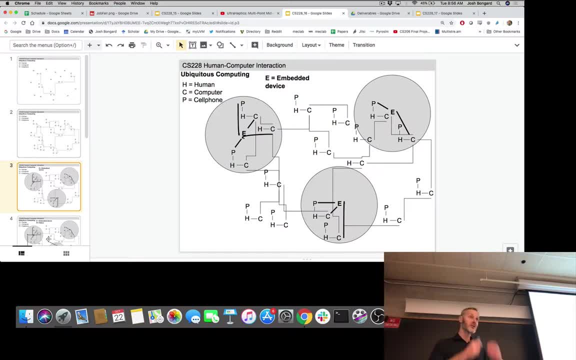 few lectures to look at embedded devices. so these are devices that also have a lot of sensors and are also direct, interacting directly with some field of view around them. a simple example would be the motion sensors over in the davis center. the sensors themselves don't move, but they 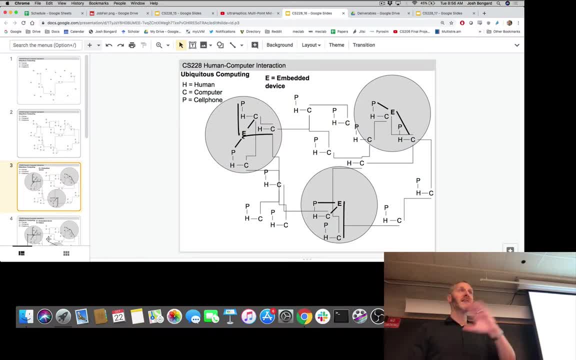 sensing in real time something about the real world, independent of whether there are people around or not. and towards the end of this section on looking outward, we're going to look at robots which, from an HCI perspective, are nothing more than self moving embedded devices. robots over embedded devices are able to push. 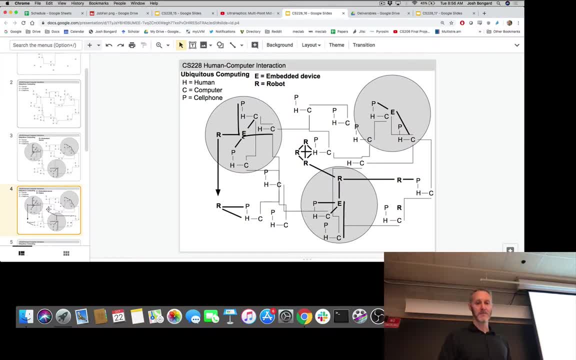 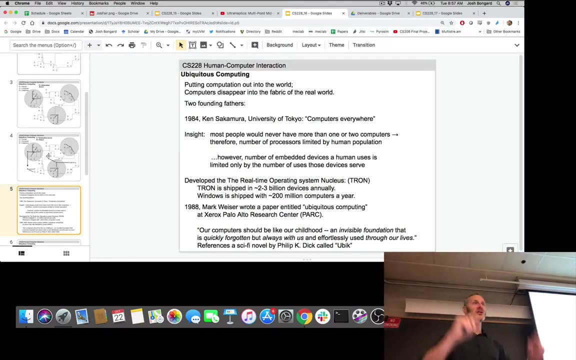 against the world and observe how the world pushes back. okay, so this is the world that we're moving towards and there are some important HCI challenges and opportunities in doing this right. that's what we're talking about in ubiquitous computing, which you can think of as putting computation out there into 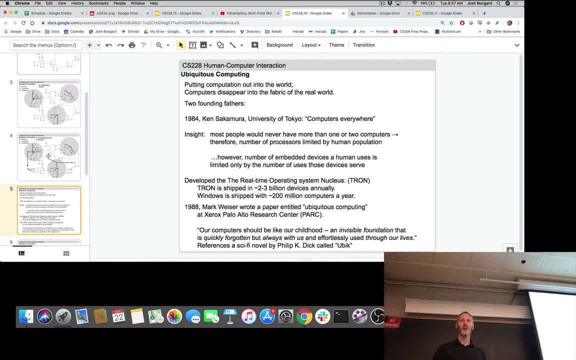 the world, and if we do it well, the technology disappears into the world. how many CPUs are there in this room right now? a lot, that's a good guess. who knows right? hopefully I'm. luckily, we're all not aware of each other's cell phones. we know they're out there. 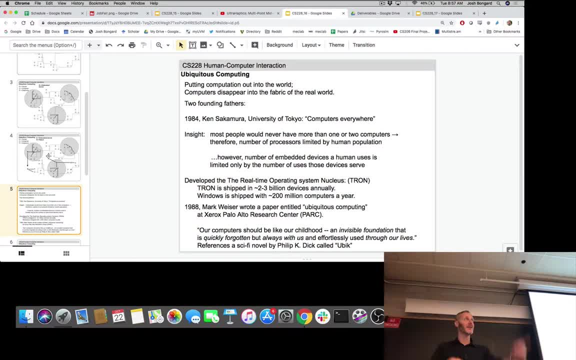 there's a bunch of CPUs out here, there's one in here, there's one in there. it's out there and a lot of those CPUs are doing active work for us at the moment and are helping support this activity of learning about ubiquitous computing. but hopefully, most of the time the technology is not you're not aware of. 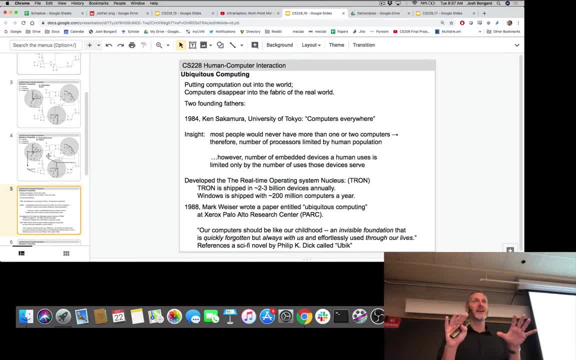 the technology and instead you're resting on that technology and using it to learn about ubiquitous computing. how do we create ubiquitous technology that is invisible? this is an idea that goes way back to the early 1980s. Ken Sakamura at the University of Tokyo was one of the 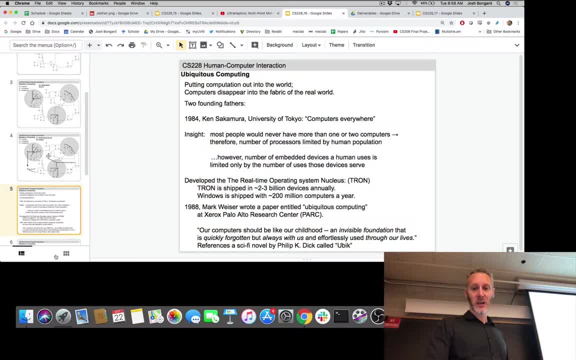 founding fathers of ubiquitous computing, and he wanted to put computers everywhere. even back in the 1980s, when personal computers were just getting started, Professor Sakamura had the insight that even if every single person on the planet bought a desktop and eventually a laptop, we're probably not going to have 10 or 20 computers. 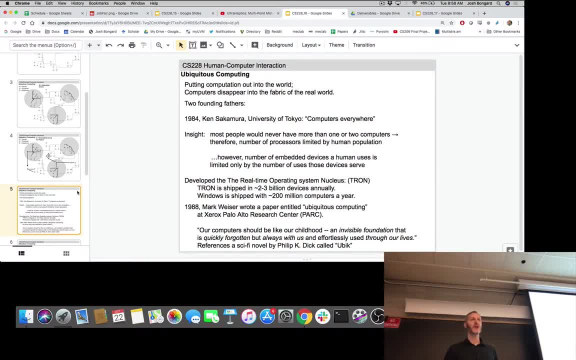 but we may have many, many more devices which are computerized. this was a pretty insightful observation way back in the 1980s. so the number of embedded devices a human uses is limited only by the number of uses you can think of them. so inside your laptop there are a number of CPUs in your day-to-day life. among the 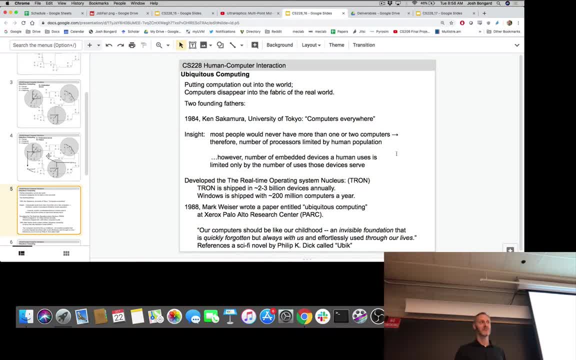 objects that you own. where else are there CPUs, everything: your car, your phone, kitchen appliances, absolutely Wi-Fi router. okay, if you have a laptop, you're running- you're running Mac OS or you're running Linux or you're running Windows- what are all those other CPUs running? a lot of them are probably. 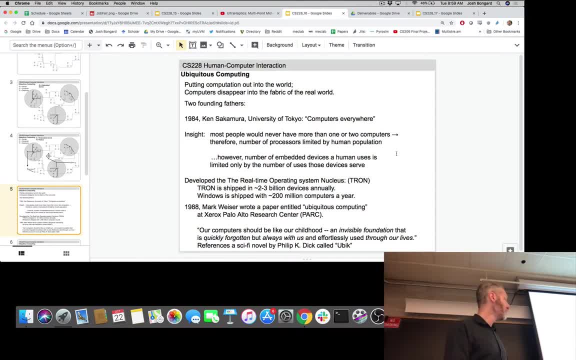 running the real-time operating system Nucleus, Nucleus memorably known as Tron. how many of you have heard of the Tron operating system, couple of people? it is the most popular operating system on the planet, at least as of last count. thanks again to Professor Sakamura, okay. 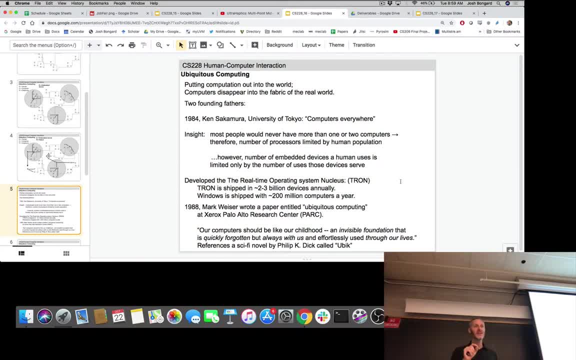 we're not going to talk about Tron itself. the point here is that among advanced computer science students we're not even aware of the fact of all of these devices and the operating systems that their running. hopefully those devices are in the background and are helping you drive to drive. 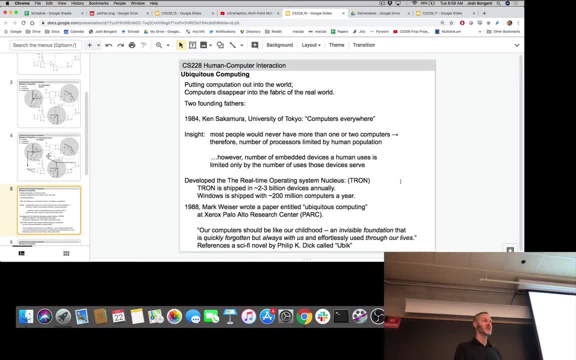 to campus in the morning helping you prepare meals and so on. they're in the background and they're because they're working. well, they're invisible. mark weiser at the xerox palo alto research center, known as park- this was the google of its day back in the 80s and 90s- coined the actual. 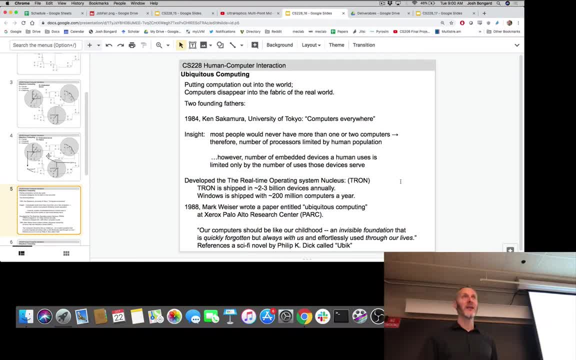 term ubiquitous computing. ubiquity means sort of everywhere, and mark was the one who wrote our computers and he meant here. ubiquitous technology should be like our childhood: it's an invisible foundation that we rest upon. that's quickly forgotten after you learn about it, but it's always with us and effortlessly used throughout our lives, and we can call it into. 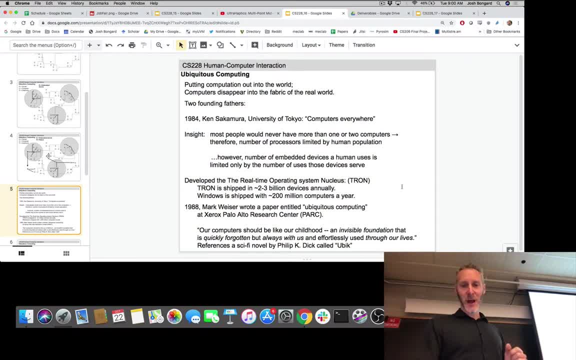 the foreground when needed. he was inspired by the name from one of philip k dick's novels called ubic. if you're a science fiction fan, i highly recommend this book. okay, so that's the idea of ubiquitous computing which helps to orient us to think about how to go about designing. 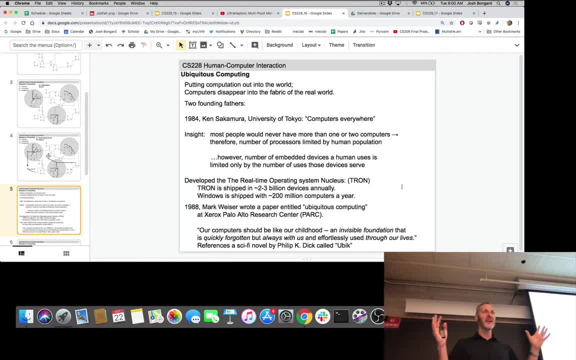 this technology. if we're going to create a large number of devices that are sensing and acting in real time in the physical world alongside us, it would be great if we're not aware of what they're they're doing. let them do their up their job so we can get on, uh with our 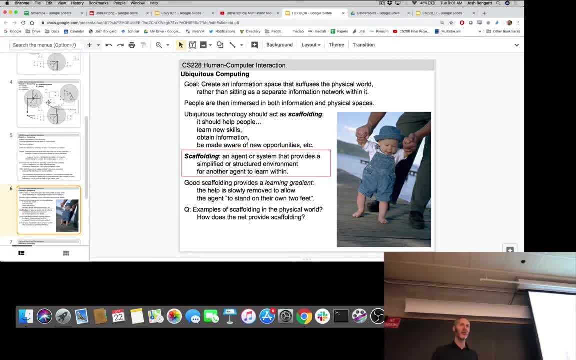 eyes. so how do you make this invisible? how do you create technology that supports us, like in our childhood? well, we're going to draw on this important concept of scaffolding and, through the rest of this section of the course, we're going to come back to scaffolding several times. 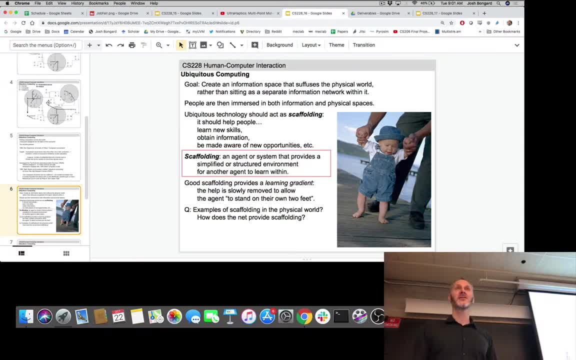 this is an idea that comes from developmental psychology or the study of child development. scaffolding is a very important and intimate process that goes on between parents and children, where parents either physically or metaphorically support the learner and as the learner starts to signal increasing competence at whatever it is they're trying to learn, which, in this case, is to 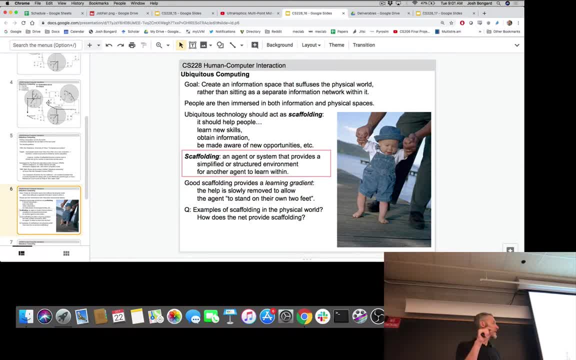 walk on their own two feet. the, the instructor or the teacher or the parent or the caregiver is sensing. the fact is somehow inferring that the learner is getting better at the task and gradually removes the scaffolding until there is none left. that's the idea. okay, tricky thing for, uh, the teacher to do. how do you detect growing competence? 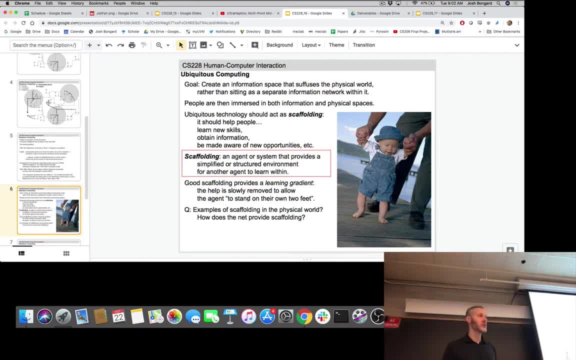 okay. if scaffolding is done right, it induces a learning gradient, so a slope up which the learner is climbing and they're getting gradually better and better at the task right. a common example of scaffolding from child development are training wheels on a bicycle, if you, if you've never ridden. 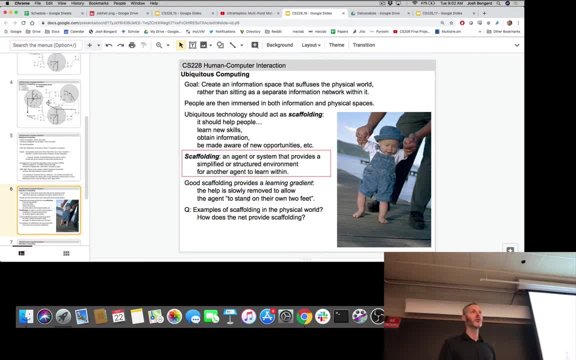 a bicycle and you get on a bicycle without training wheels, there's no gradient 99 of the ways that you apply force to the pedal pedals are going to end in disaster, and there is a very small minority of actions that the peddler can perform that will keep the bicycle upright and headed in. 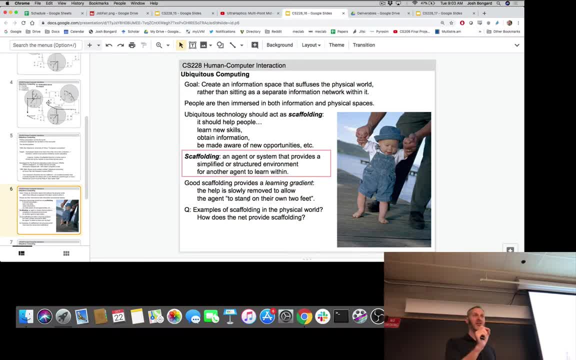 the right direction. how do you find that action, that needle in the haystack, if everything you do causes the bicycle to fall over? you add training wheels and now the peddler can perform a certain, And now 50% of your actions cause the bike to move a little bit forward. and the rest? 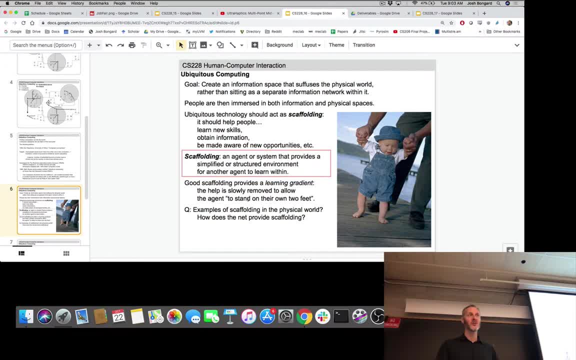 cause the bike not to go anywhere. There's now much more opportunity for the learner to start to experiment with this device and learn about it, and when they finally figure out how to induce motion and balance on the bicycle, you can remove the training wheels. 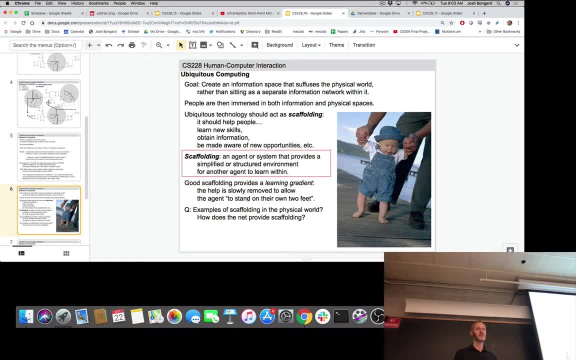 What are some examples of technology that do something similar? Any new software that usually pops up with tips. so when you're learning it it asks you if you want tips or if you're an advanced user- Absolutely right. So a lot of software at the beginning says: do you want to be walked through the tutorial? 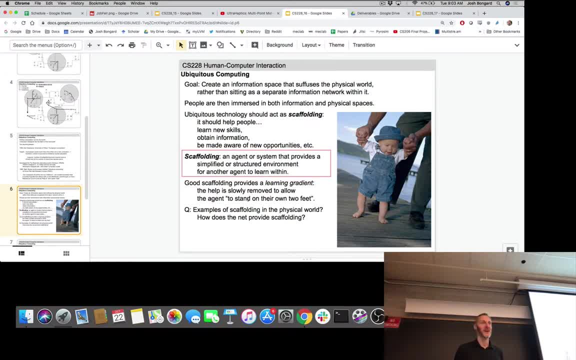 or the tips And you have to click on something to say yes or no, which is fine. but now obviously we've cost the user having to click and say yes or no. Good technology doesn't have to ask the user, but like a good parent, it's still. 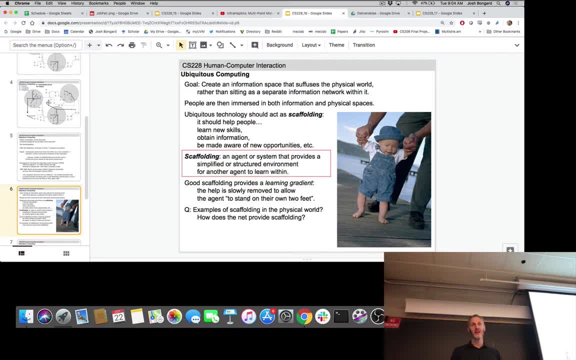 sensing growing competency in the user and removes scaffolding and tips and tutorials as competency increases. I feel like Clippy could have been like a temp at scaffolding. Clippy- Good old Clippy right- Failed miserably at this task. But it doesn't require you to ask for help, but it will come and say it will figure out. 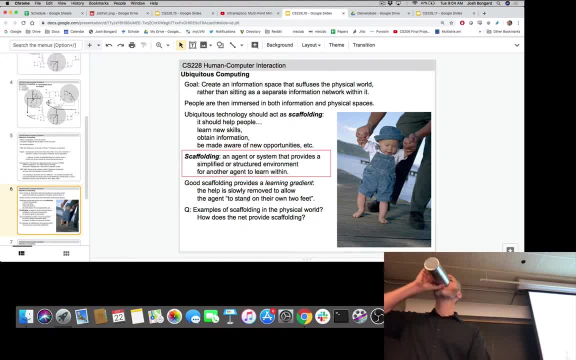 that you're trying to do something and maybe struggle with it, Absolutely So a lot of technology, if it senses that you're struggling, will pop something and ask if you need help, which is Okay. Other examples: Okay, Let's try and, for a moment, mentally design some technology to do the scaffolding. 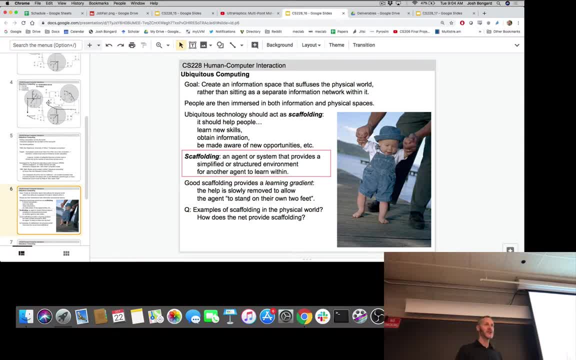 You've all probably used GPS on your phone. You turn on GPS and it tells you how to get from point A to point B. If you turn on sound, a voice tells you: in a thousand feet, turn left. In 500 feet, turn left. 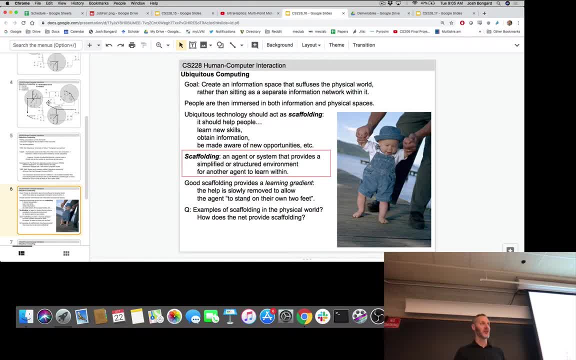 In 250 feet, turn left. If she tells me one more time to turn left, I'm going to throw my phone away. I'm going to throw my phone out the window. right, It's all good, It's fine, But could you imagine a GPS system which is sensing growing competency? 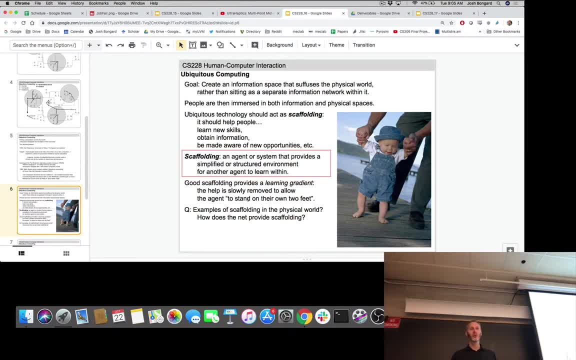 So I trace the same path a couple days in a row. What is it that is going to tell the GPS whether I've remembered the route and I don't need to be told anymore to turn left, Or I was talking to a friend and I wasn't paying attention the last time we traced this? 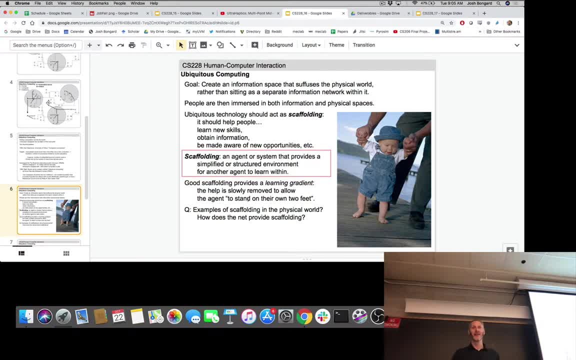 route, so I still don't know how to get from point A to B. I'd like some verbal help. Of course GPS could ask and I could say yes or no. but could it infer growing competency? How would a GPS system know whether I'm learning the route or not? 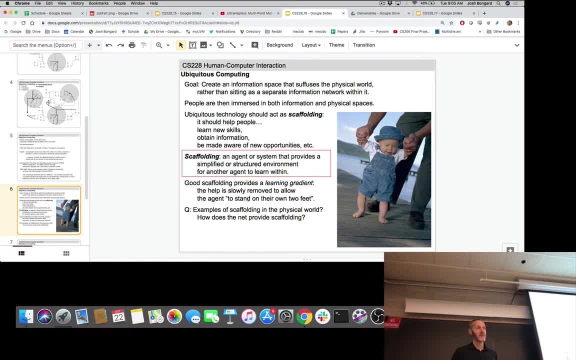 You can sense the car's speed, the speed of the car. So we have an accelerometer in the phone. This is probably going to be useful. but how does acceleration, what features of acceleration, will tell the GPS system? Yeah, Acceleration will tell the GPS system whether I know the route or not. 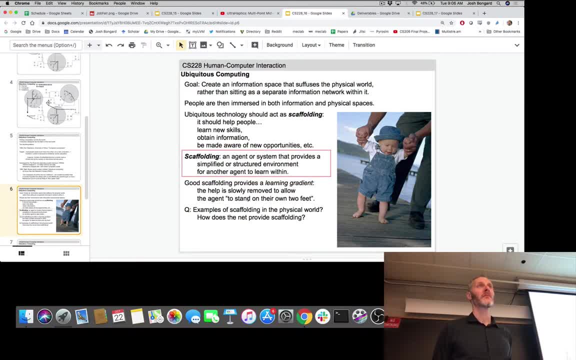 Maybe a certain change in speed and then a signal, and then an anticipated trend, Okay, A kind of a narrow, a wind, and then a- Exactly, We're getting closer right. Something, a change in speed, which is, by definition, acceleration, might be able to. 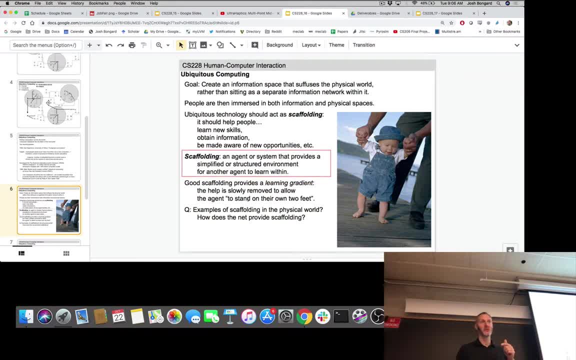 tell the system that I know I'm going to turn left soon or not, but it's tricky. What feature of acceleration might tell you that? Well, if there's any indication that the GPS voice would have an effect on your speed, that would mean that 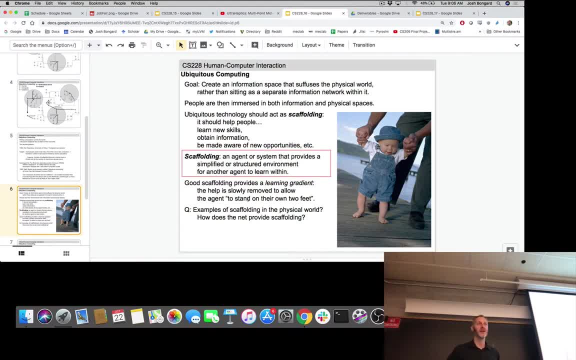 There's a great example, right. So perhaps she asks a probing question and it causes me to change my acceleration. If she's giving verbal hints and I'm ignoring her and when she speaks my acceleration does not change, That's a sign that maybe I know the route and I don't need any more verbal hints. 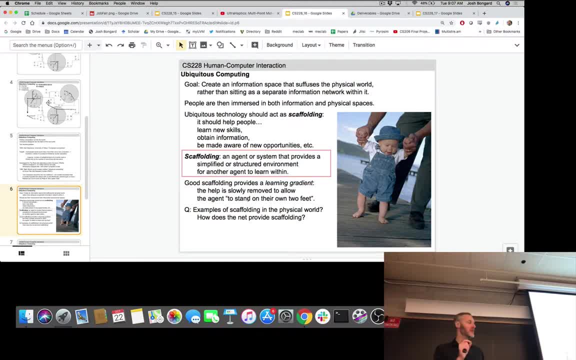 That's a great observation right, Paying very careful attention to, in this case, the physical context of driving, either aided or unaided by a GPS device, and using that to allow the GPS system to remove scaffolding when it's no longer needed. 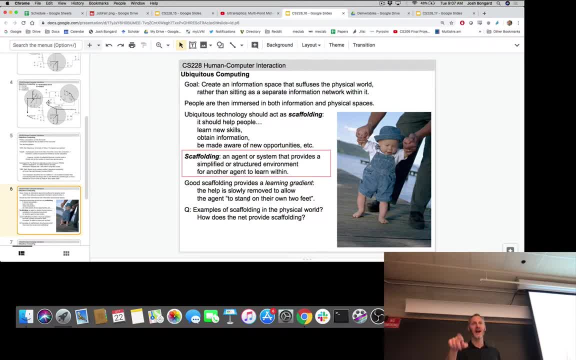 Because, especially in a driving situation, I prefer not to have to look down at my phone and turn off or mute the system. Okay, That's the sound, Right? It would be good if this was just intelligently inferred. Absolutely Right. 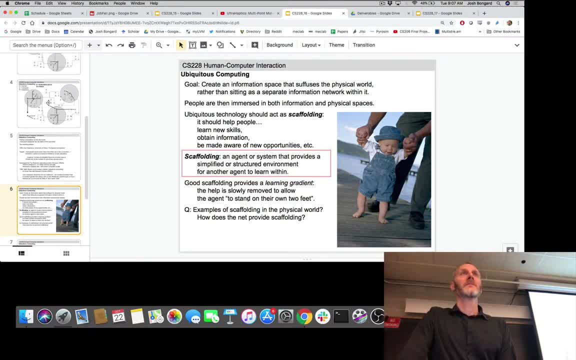 So we could start to use facial recognition, lots of other features going on in the car that we could exploit to figure out how to intelligently tune the amount of scaffolding provided during route taking. Okay, So, as I mentioned, we're going to come back to this idea of scaffolding several times. 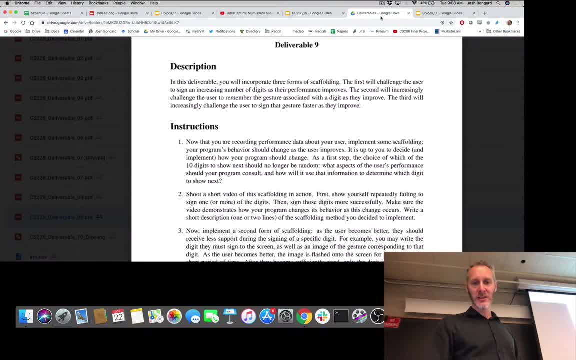 throughout the rest of the course, and scaffolding is the focus of Deliverable 9.. In Deliverable 9, you're going to be adding three scaffolds to your system. educational software in particular, or education is all about scaffolding. 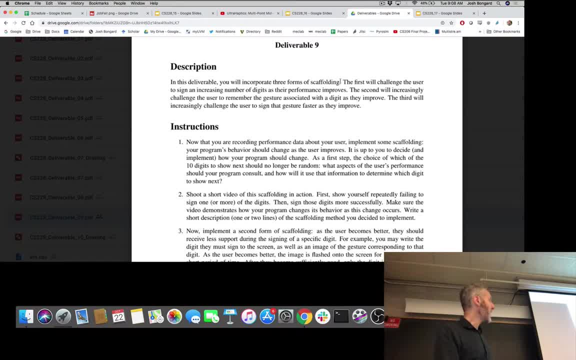 First scaffold you're going to be applying is challenging the user to sign an increasing number of digits as their performance increases. So instead of creating a system that says: I think you're pretty good at digit zero, Would you like to move on to digit one? 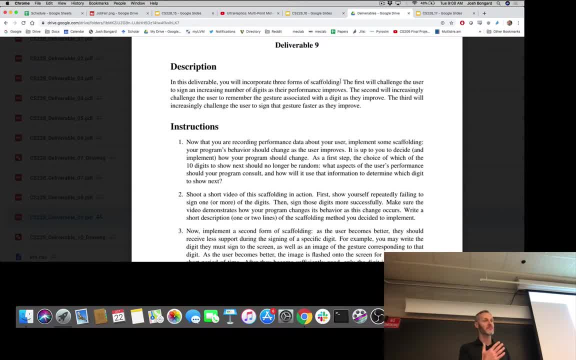 We're going to try and intelligently infer increasing competence and expose the user to more digits as their competence increases. How can you detect increasing competence, given your code base so far? Choose the number that's accurate, right? Yeah, Yeah, Yeah. 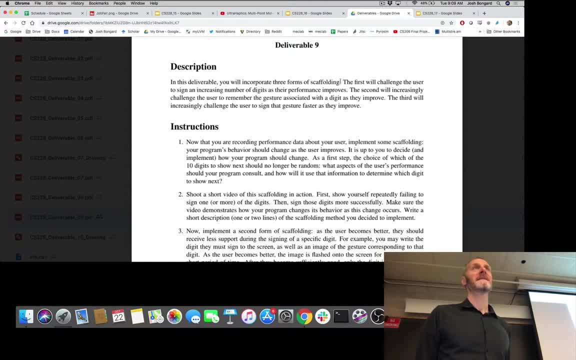 Yeah, Absolutely right. So your KNN is going to come in very handy here. Your KNN will be able to tell you whether the user is signing correctly or not. We might average over multiple demonstrations and take some average. Is the average number of correct gestures increasing? 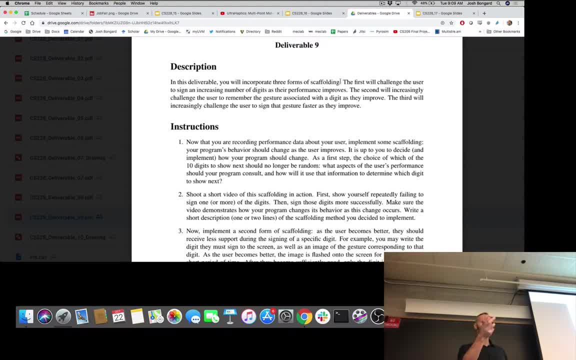 Like the example of GPS Right we just talked about, there's some other additional subtle cues that you might be able to pull out that indicate growing confidence, exactly absolutely so. time is going to be very important as we move forward with this technology. I can't. 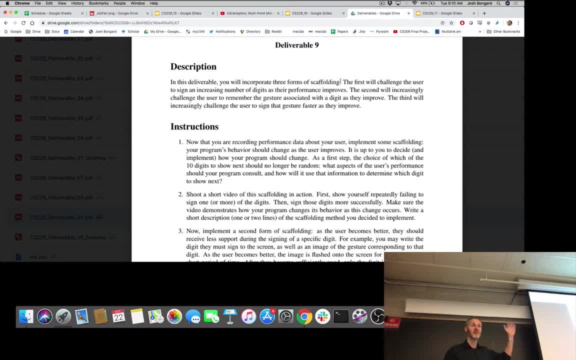 remember if we've introduced the time library yet or not. if you haven't, it's very useful. you could measure, using the time library, the number of seconds that elapse between your system, flashing up the digit 3 and the number of seconds that elapse until the KNN detects or predicts that the user is signing the. 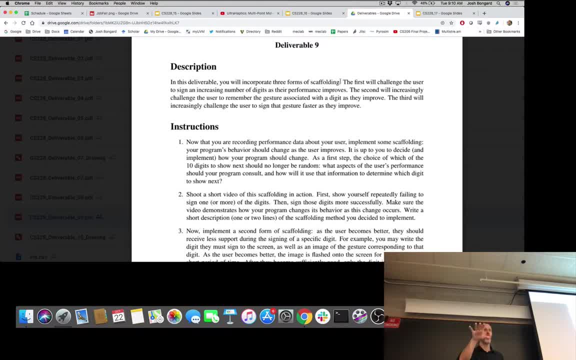 digit 3, how long does it take the user to figure out what to do? in addition to, how often do they get it right? so there's a double challenge and deliverable 9, which is not just thinking creatively. but it's a double challenge and it's not just thinking creatively. 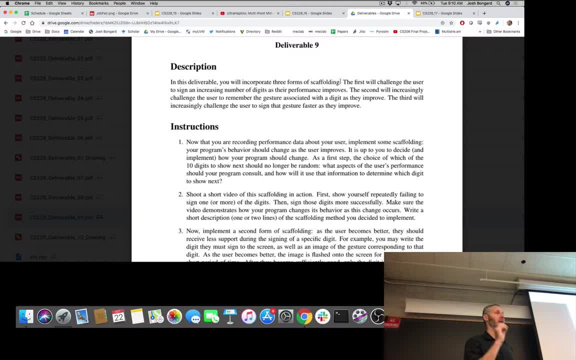 about the scaffold itself but, more importantly, knowing when to apply the scaffolding and when and how to gradually remove it. okay, second scaffold you'll be adding will increasingly challenge the user to remember the gesture associated with the digit as they improve. so at the beginning we're 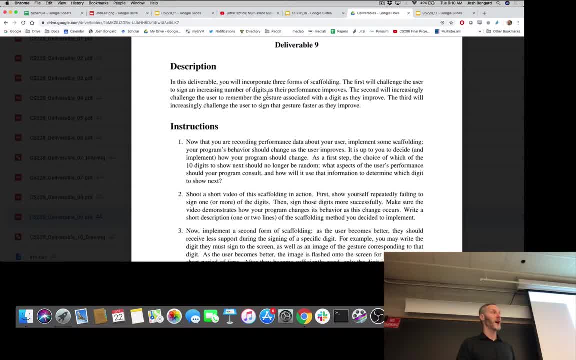 going to tell the user how to sign 3, 4, 5 and so on, but we would like to gradually remove the scaffolding as we go forward, of showing them the gesture and forcing them to remember it. simplest way to do that is obviously to flash up an image of the gesture itself for a shorter 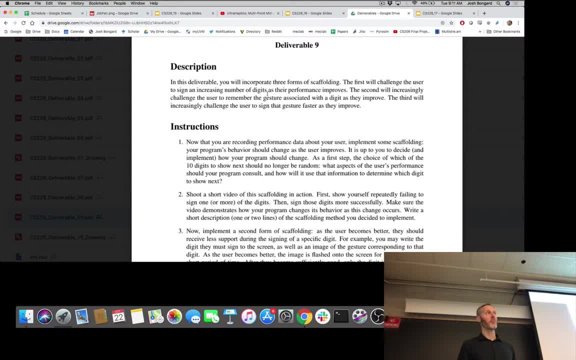 period of time. how else might we help our users gradually memorize the gestures associated with the digits? one of the one of the challenges and scaffolding is not to remove the scaffolding immediately. take off the training wheels and now we have a learner that's completely unaided. we're 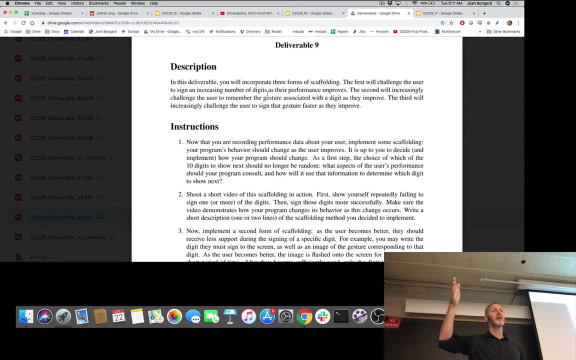 always looking for ways to include gradients to make this process of learning or memorization, in this case, as smooth as possible. the gesture: we have the image of the gesture. the image or a figure, whatever it is, you're showing the user what they should do. you can remove it after a shorter and shorter period of. 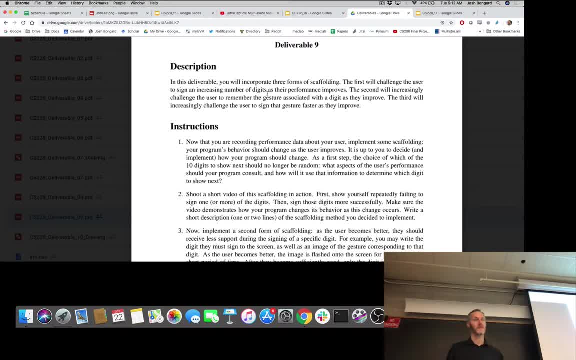 time. what else could we do? absolutely, you could. we could put up an image of the gesture, but you also have the virtual hand itself. you could draw the virtual hand that corresponds to whatever the user is actually doing, could draw an additional skeletal hand which is showing what they should be doing and they are trying to match their 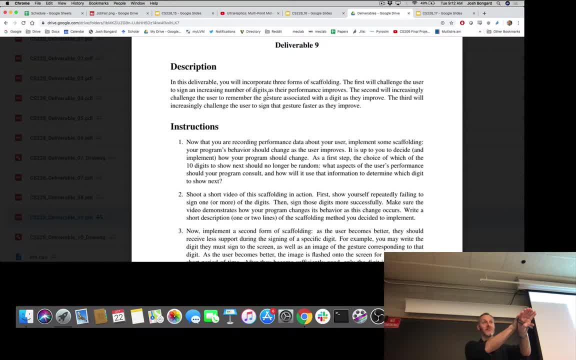 visual hand with the demonstrated hand. okay, so go from do this to pick which of the two is correct. so recognition rather than remembrance. we talked about that several times already. I three and six. I still get confused after all these years. if you put up two images, I can usually 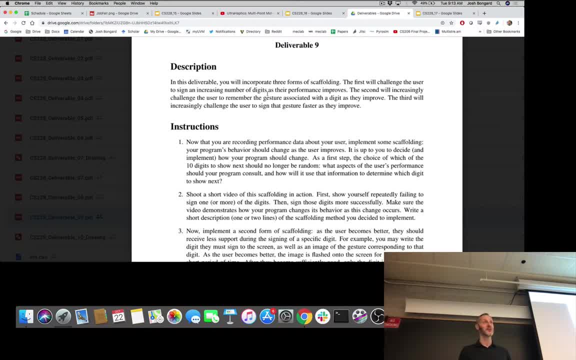 remember which it is. unless the two images are three and six, then I'm still confused. but I can usually pick up the sign for three compared to one, compared to one or zero and so on. so we could go from do this to challenging our user to recognize and then finally to challenging them to 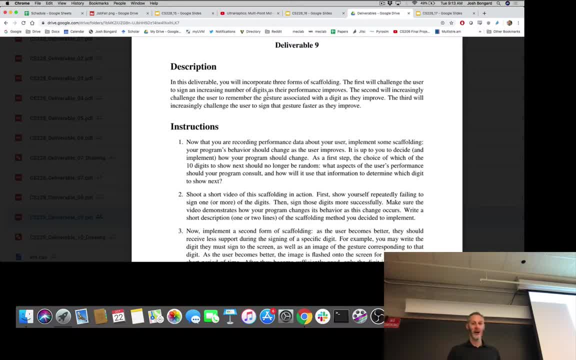 remember right, that would be adding in a gradual learning gradient. okay, again, in this assignment and all the rest of the assignments, it's up to you to come up with your particular solution. the third scaffold will increasingly challenge the user to sign that gesture faster as they improve. how might you induce a learning gradient here? okay, okay. 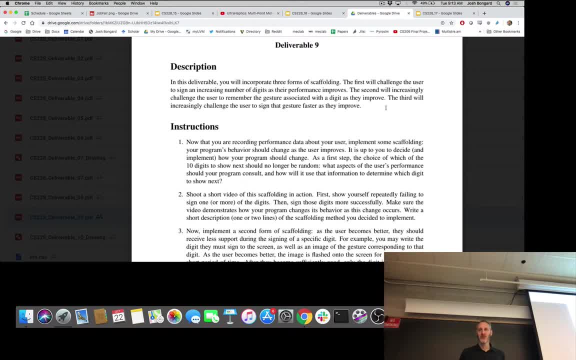 there's a great idea, right? if you get into sequences of numbers and you need to sign them as quickly as possible, maybe the sequence grow the longer as, again, they're able to succeed in this, this task. okay, any questions about deliverable nine? it's pretty straightforward, okay, okay, so that. 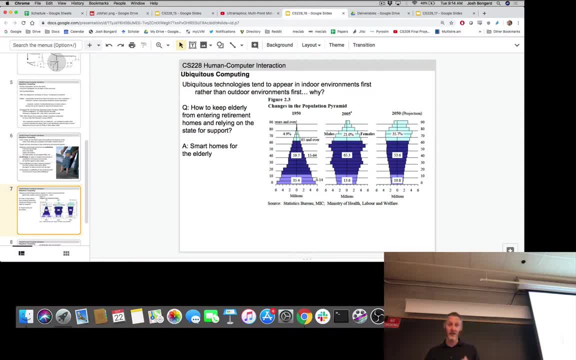 scaffolding. let's have a look at another application. this one is is one of the primary applications of ubiquitous computing. another reminder here of visual design. what are these three population pyramids? on the right telling us populations are getting older. right, the graying of the global population. these 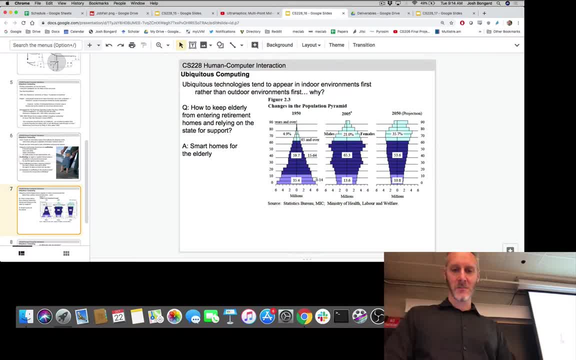 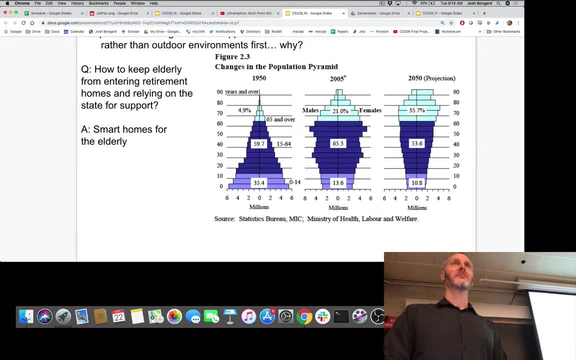 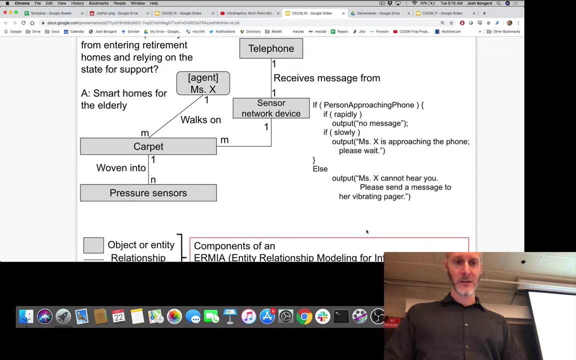 are three population periods at three different points in time for a particular country. which country is it United Kingdom? very good, how did you know? thank you, the Ministry of Health and Labor spelled properly. ok, ok, so one of the challenges, obviously, in manipulating slides, which I'm clearly- 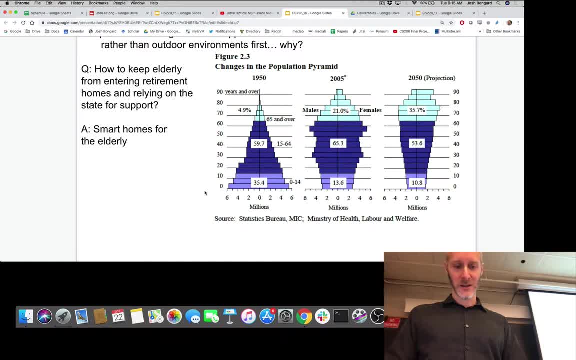 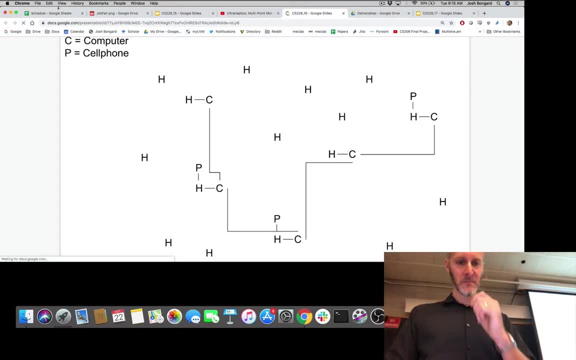 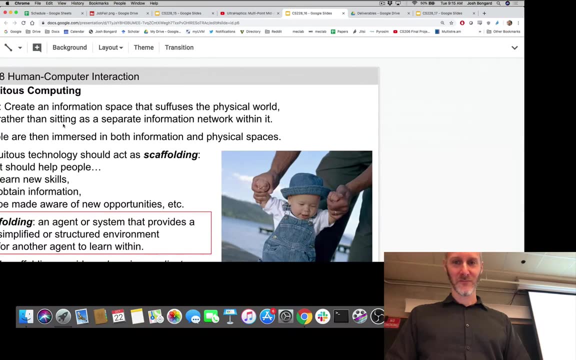 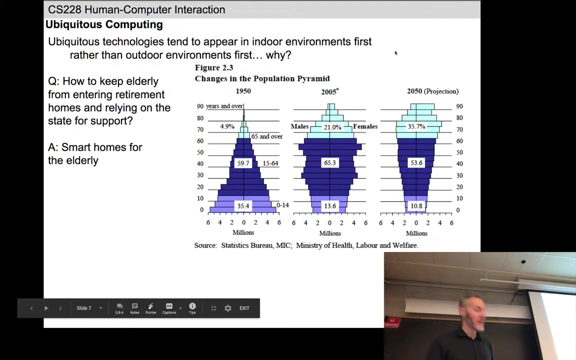 not very good at how do I. that's not going to help us much. let's try this. let's try this, ok, ok. so We're going to look at an application where we're going to think about trying to deploy ubiquitous technology into the homes of the elderly so we can keep them as independent as possible. 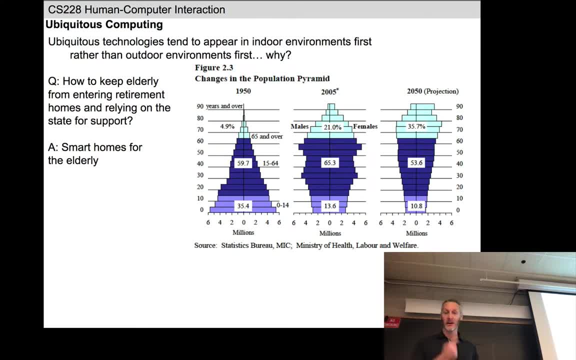 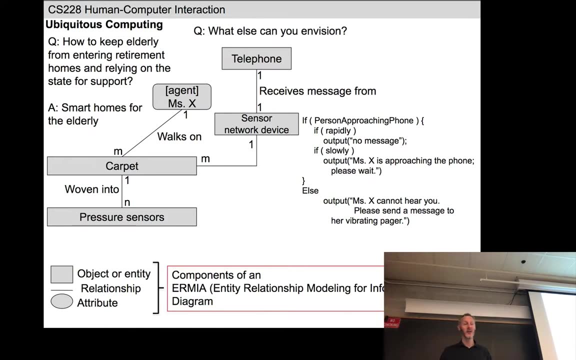 Most people would prefer to stay in their homes than in a care facility, and from an economics point of view this is also useful for from a social point of view. So here's a little cartoon example. here We have Miss X who lives alone in her home and her mobility is declining. 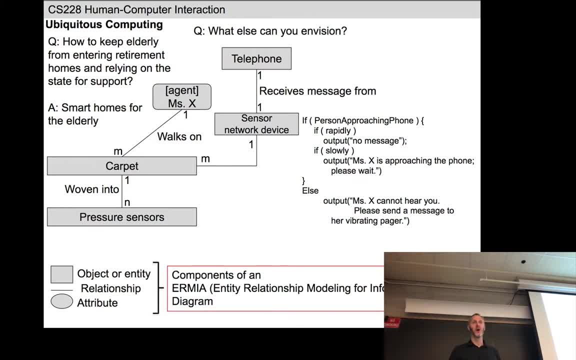 Family members would like to call and check in with her every once in a while. If you call and the phone keeps ringing, do you jump in your car and drive over, or is everything okay? One potential application would be to stitch a number of sensors into various carpets or flooring. 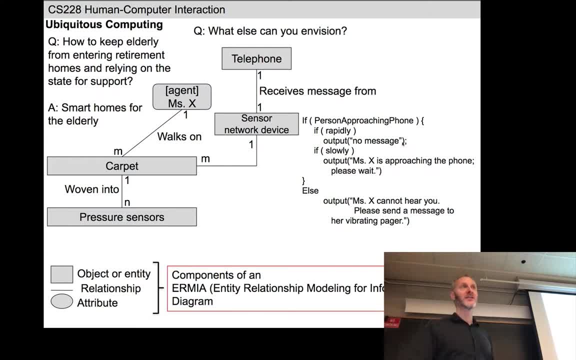 throughout the home And write a little bit of code to support this distributed sensor network. If the phone rings and we detect pressure sensors- we detect pressure on the carpets and it's Miss X moving about, We give a message saying Miss X is approaching the phone. If she's almost at the phone, just let the phone ring normally. If the 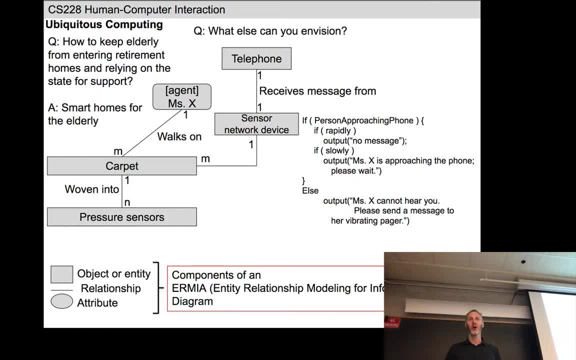 phone continues ringing and there is no detection of movement in the home. perhaps you send out an alert to the care camera. I've drawn this using something known as ERMIA, or entity relation modeling for information artifacts. It's a bit of a mouthful, but if you work in industry you'll probably come. 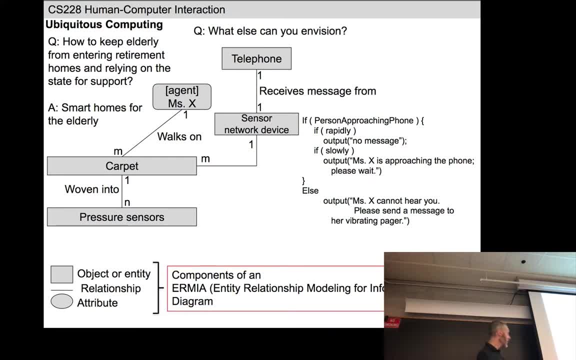 up against the ERMIA notation. In ERMIA notation, we're going to use rectangles to represent physical objects in some way. They could be people, they could be non-intelligent devices, they could be intelligent devices. We can have attributes associated with those devices. We can draw edges to connect together objects. 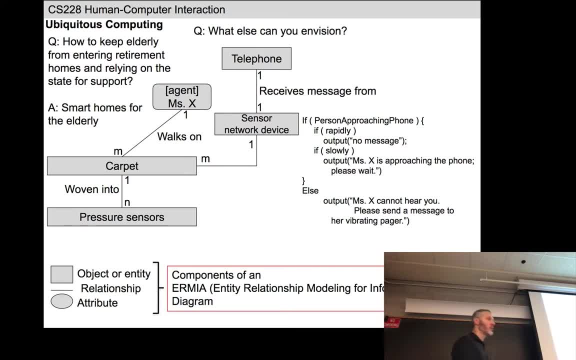 And numbers in the corners of connectors represent the one-to-one, one-to-many or many-to-many relationship. So in Miss X's home she has M carpets and in each carpet there are N pressure sensors. Again, this is a little bit cartoonish. It allows us to pretty quickly sketch out an idea. 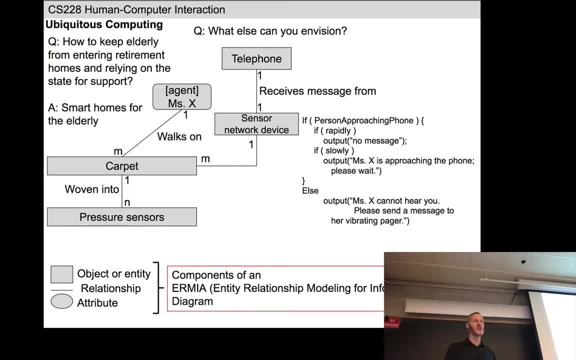 for a distribution: people, objects and technology. What else might we deploy into Ms X's home to increase her independence, Assuming that she is challenged by decreasing mobility? Any ideas? What's the context here that's most relevant? Maybe motion detection, Motion detection- Okay, so we're trying to detect motion. 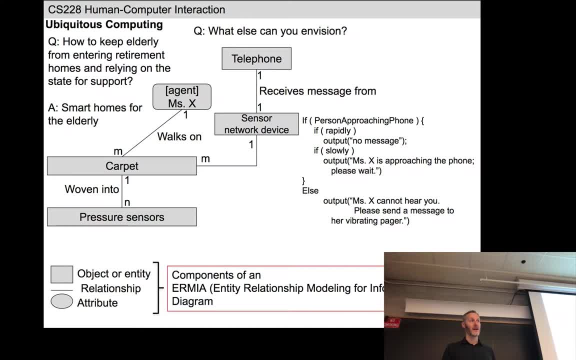 Yeah, see Mrs in which house and how she moves. Okay, so maybe motion detectors in the rooms to detect motion. Okay, so maybe motion detectors in the rooms to detect motion. If we want to detect Ms X's motion, what's the easiest way to do it? 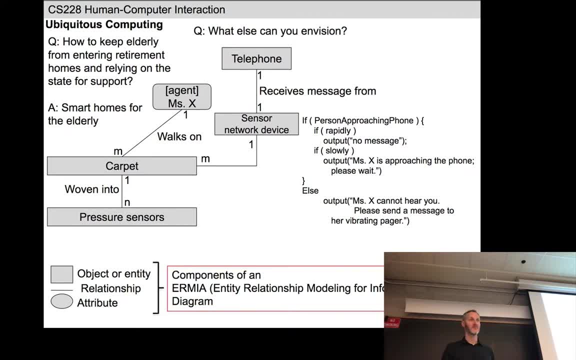 Have a wearable sensor. Maybe Ms X is not willing to wear that technology right. The easiest solution to keeping people independent in their homes is to turn their homes into Big Brother. right Sensors everywhere, on the person, in the person. in some cases, However, again, that may be the most that might be. 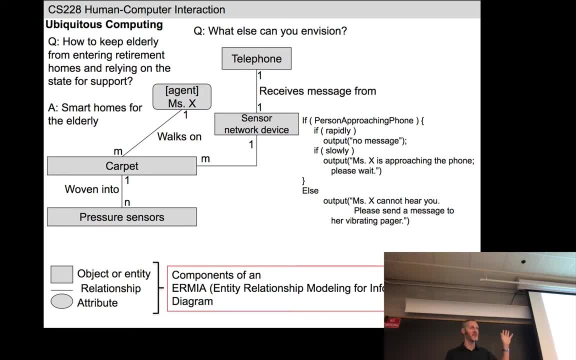 the easiest way to solve the problem, but from Mrs X's point of view, it may be unacceptable. right That someone is watching at all times. Again, we've talked about acceptability. This is a difficult thing to get right in this domain, but 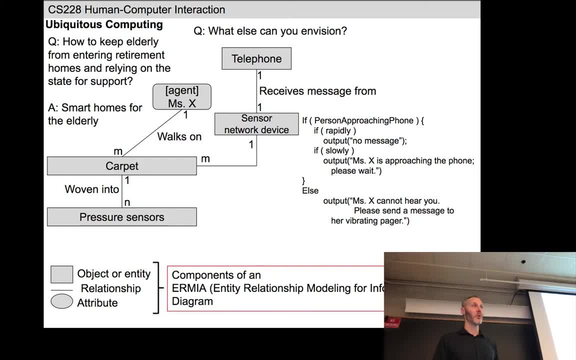 again, from a health care perspective, very, very important and increasingly important. Okay, thanks, Okay again, just something to think about. Okay, Lecture 16 is a little short, so we're going to move on now to Lecture 17.. 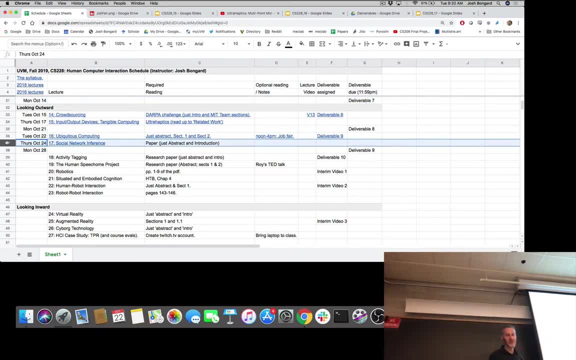 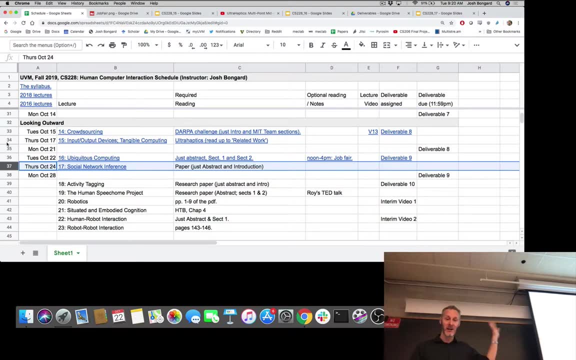 In Lecture 17,. we're going to look at the first of these three applications where we're going to try and apply ubiquitous technology. We're going to look at some investigators that deployed ubiquitous technology to pose and try and answer a scientific question that would be difficult or impossible otherwise. 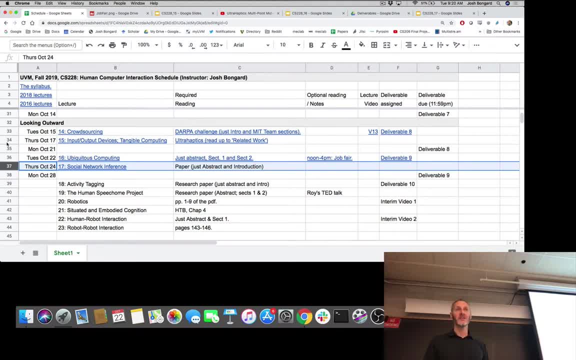 The first one we're going to look at is social network inference. So if you give me all your Instagram accounts, I can use those to know your social network, at least that part of it that's on Instagram, Assuming I don't have access to your social network. 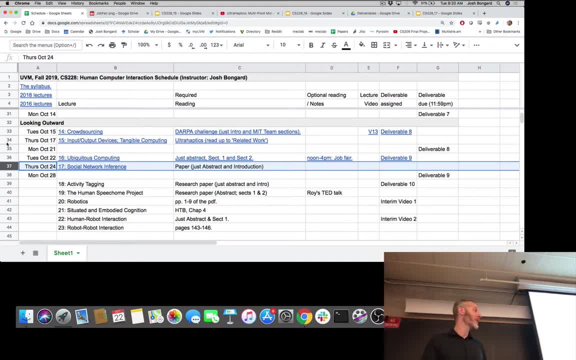 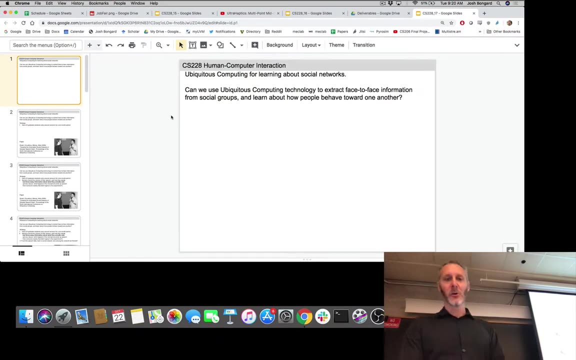 and I just interact with you physically, in an informal manner on campus. how might I infer the social networks that exist among this class? Let's have a look at an application of this. In this case. the investigators wanted to ask the following question. 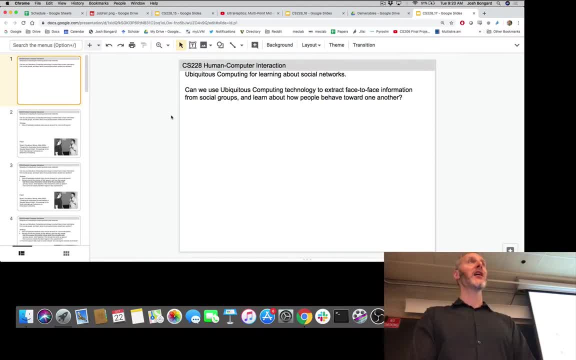 Could you use ubiquitous computing technology to extract face-to-face information? So not tweets and Instagram posts, but look at face-to-face information from social groups and learn about how people behave towards one another in this social network. Okay, that's the starting point. 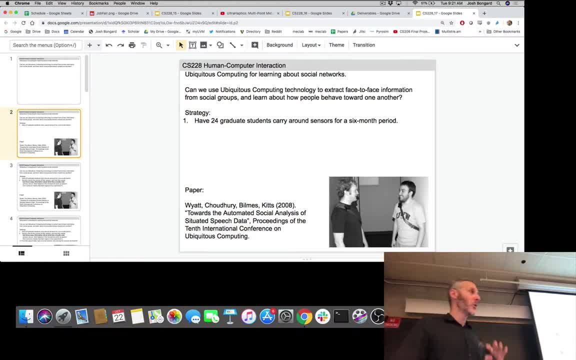 Let's talk a little bit about the experimental design. We're going to just talk about this at a high level. for those of you that are interested, You can go and have a look at the research paper itself. There were 24 graduate students who were not involved in the study. 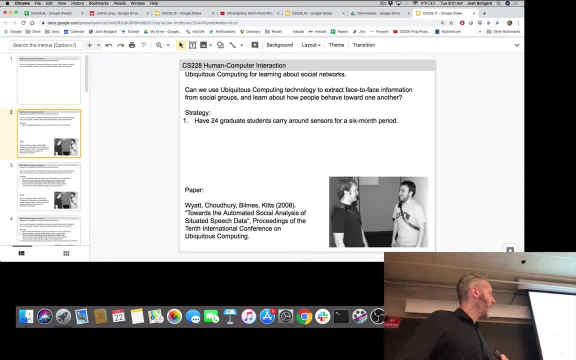 They were graduate students from a different lab. These were very accommodating graduate students. They were willing to wear back in 2008,. this sensor pack which you can see, is on this strap going around the back And, tellingly, this sensor array is close to the speaker's mouth. 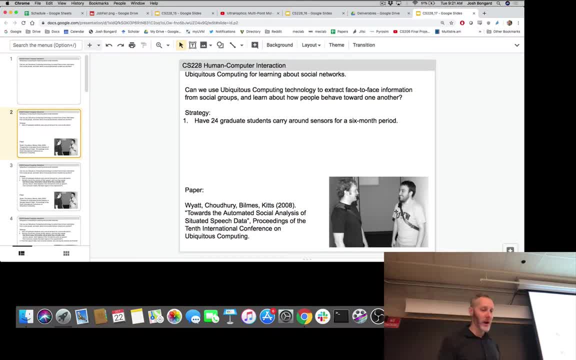 and also to the speaker's mouth And also close to their ear. They agreed to wear it for a six-month period. The sensors recorded what the speakers spoke, but it threw away all the information of the content of speech. We're going to see this several times in many of these applications. 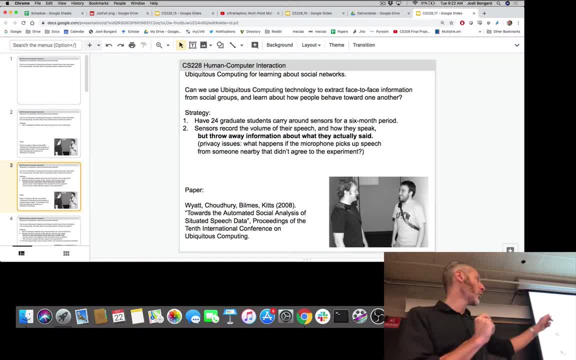 For important privacy reasons, we are not going to be recording what the person wearing the sensor said, what the person they were talking to said or, most importantly, a third person walking by who knows nothing about this application or this project. It's also not going to record what they said. 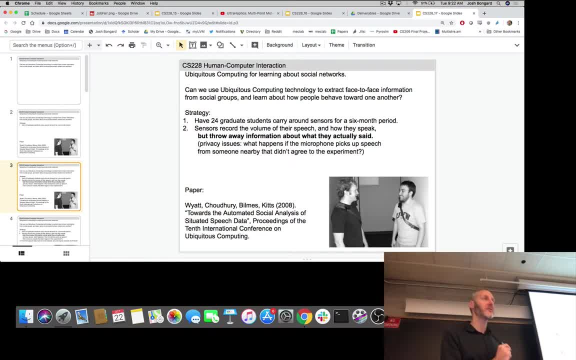 We're going to just record, in this case, the volume of their speech and what's known as prosody, the way in which they spoke, And we'll talk more about prosody in a moment. Okay, Given this speech data, we're going to collect how people spoke. 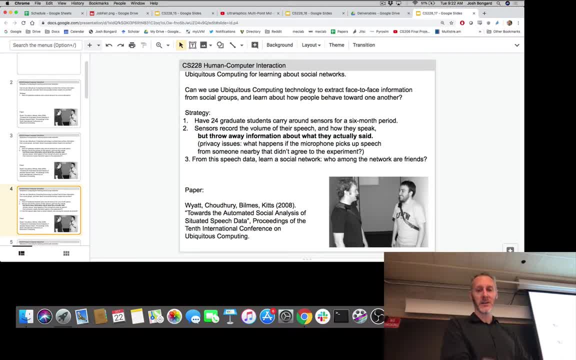 how these 24 people spoke over a six-month period. can we infer from that? first of all, can we learn a social network among the 24 grad students? Which grad students know each other better than others or are more friendly towards one another? 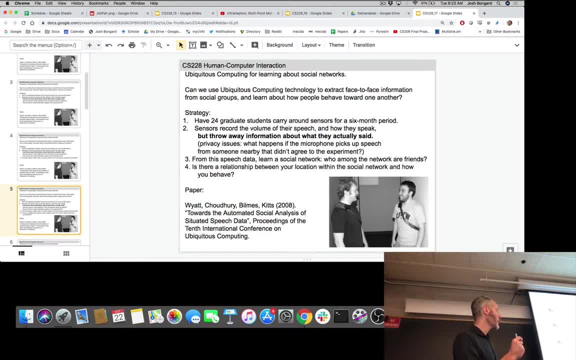 And if we can infer this social network, can we ask unique questions that would be difficult or impossible to ask in a social science setting, or questions that would be difficult or impossible to ask even if I had complete access to them, even if I had complete access to all of your Instagram and Twitter? 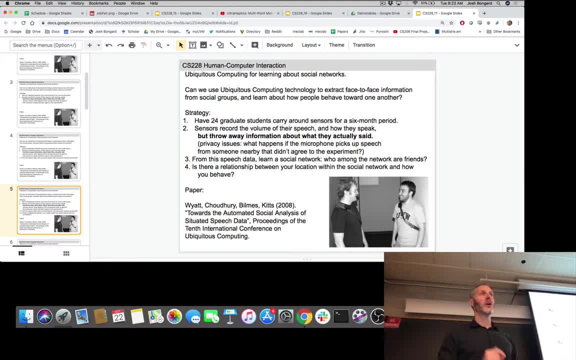 and Facebook accounts, Which is given your position in the social network. does it alter the way that you behave or the way that you speak in that network? This is a question that's been on social scientists' minds for a long time. Where are you within a social hierarchy? 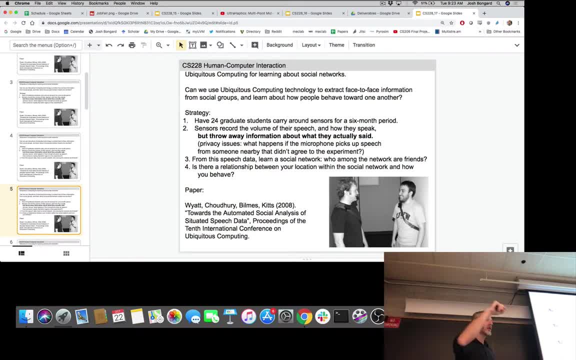 Do you know where you are in that social hierarchy And does your position or your knowledge of that position alter how you speak to others At different positions in the social hierarchy among a social group? So we're going to focus on the technology, but most importantly, 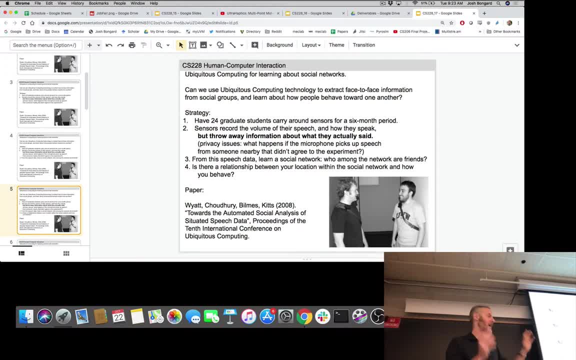 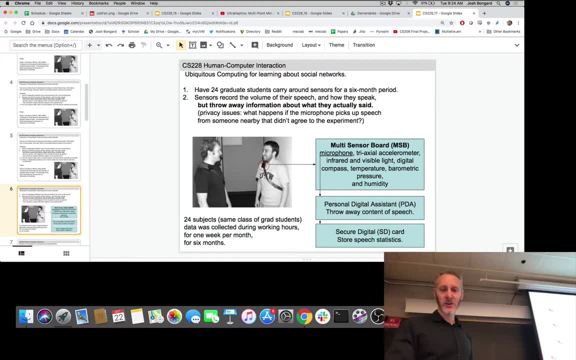 we're trying to think about how to use this technology to try and answer a question that's difficult to do otherwise. Okay, so what's in this sensor pack? There was a number of sensors: accelerometers- infrared and visible light, digital compass, temperature, barometric pressure. 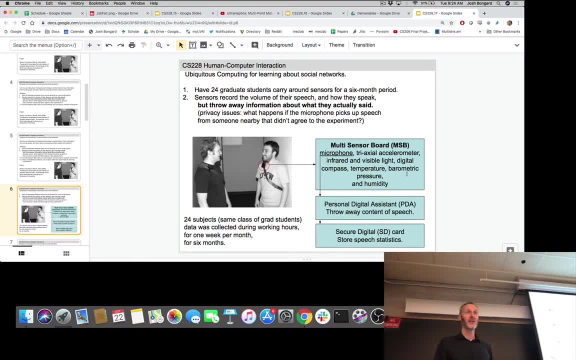 humidity, most of which probably are irrelevant to social interaction. We're going to focus on just the microphone and only focus on how people are speaking to one another, So, right at the point of capture the microphone itself, the moment that the text, the speech is captured, 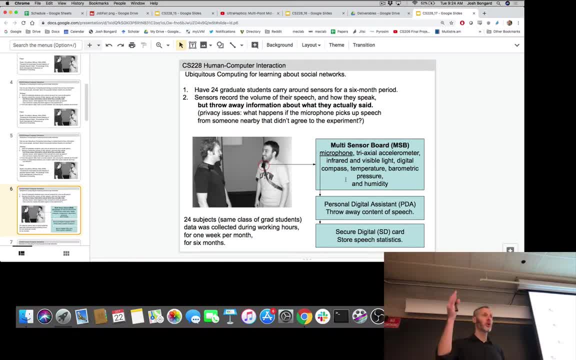 we're going to throw away the contents of speech, so that we're not recording speech, putting it on a hard drive and then throwing away the speech later. So it's an important part of the the scientists being allowed to do this experiment in the first place. 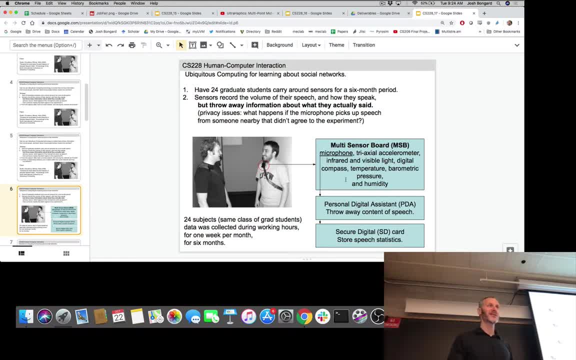 And we're going to store on the device itself just the speech statistics, the statistics of prosody, the way that they speak. Okay, Importantly, the subjects were not wearing the devices all day, every day, for six months. They were only wearing them during working hours. 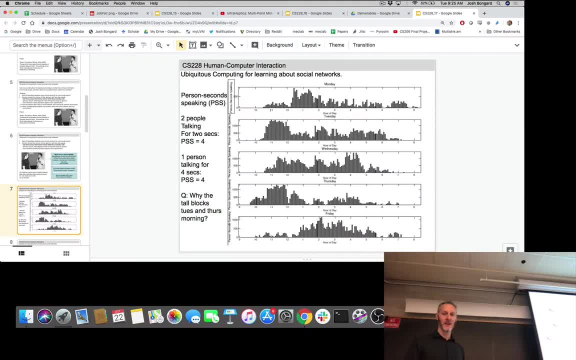 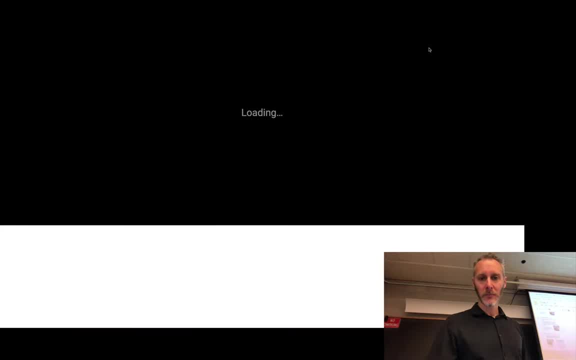 one week per month for six months. Okay, Let's dive into some of the data which maybe I should maximize this So it'll be a little easier To see. Okay, We've got five panels here which, as you can see, 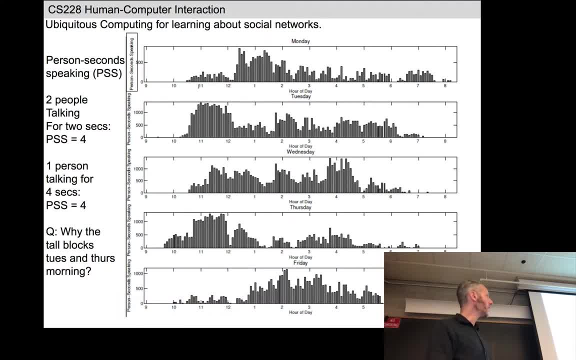 top to bottom represent the days of the working week. The horizontal axes range from nine in the morning till eight at night And in this time span we're going to break this time span into five minute buckets And inside each of these five minute buckets, 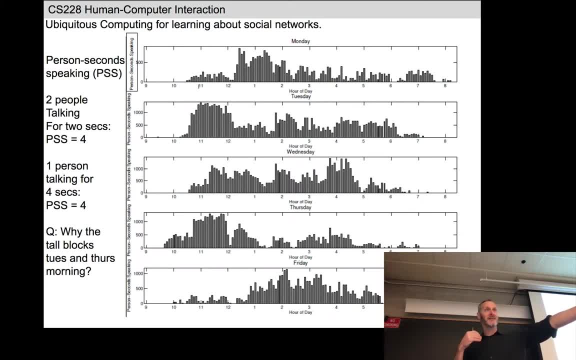 we're going to look across the speech statistics that we obtained from those 24 graduate students And within that bucket we're going to measure PSS, or person's second speaking. Imagine that within that five minute interval, all 23 graduate students are sitting quietly in the library. 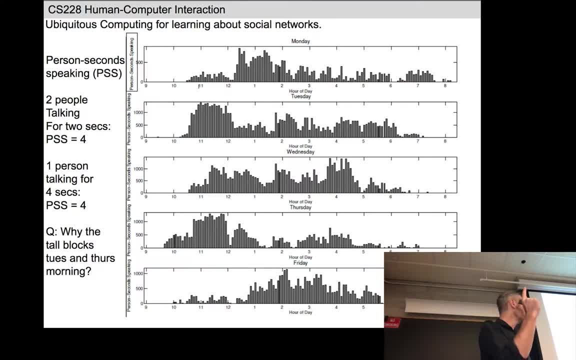 They're not speaking and they don't hear anybody speaking, but one of the graduate students is involved in conversation with someone outside this social group And they're speaking for three minutes out of that. uh, three minutes out of that five minute period. 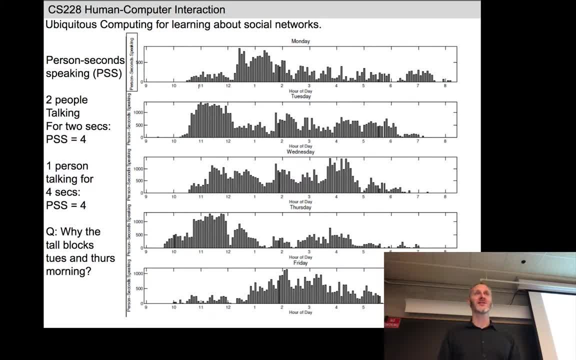 Three times 60 is 180, 180 person's second speaking seconds. Assume all 24 graduate students are speaking for 10 seconds, only 10 seconds. during that five minute period, 24 graduate students each spoke for 10 seconds, 24 times 10,. 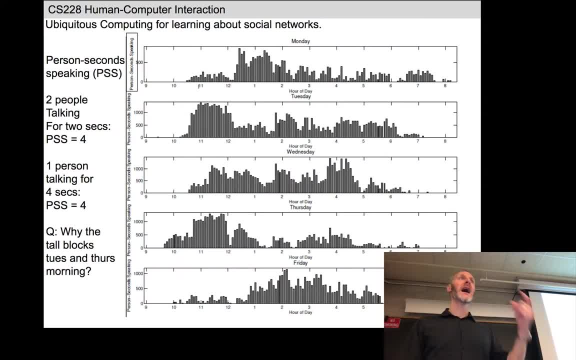 240 person's second speaking. So it's not how many people were speaking, just the total amount of speech that was going on Among those 24 students during this period. Okay, Just given that data alone, you can already start to infer something about this group. 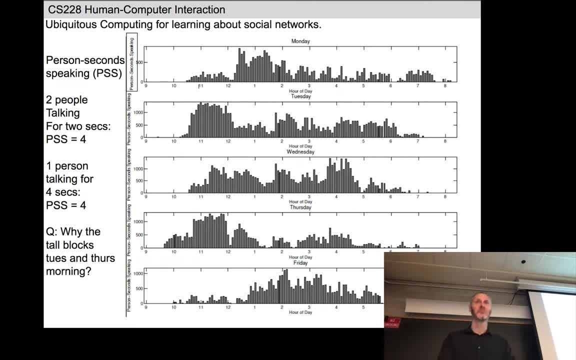 What is actually? you've been for several things about this group. Remember, as always in HCI, we're starting to think about context. right, What? what are these graduate students doing? How are they behaving? How are they speaking? What can you tell me about the context here? 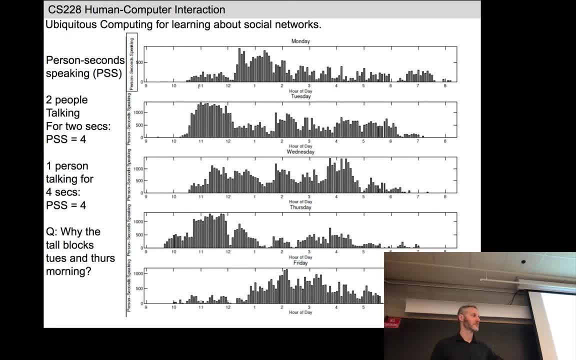 Why the tall blocks Tuesday and Thursday morning? Maybe they're in a meeting with each other. Maybe they're all in a meeting with one another, Maybe they're all in a meeting apart, but then why this regularity of Tuesday and Thursday morning? 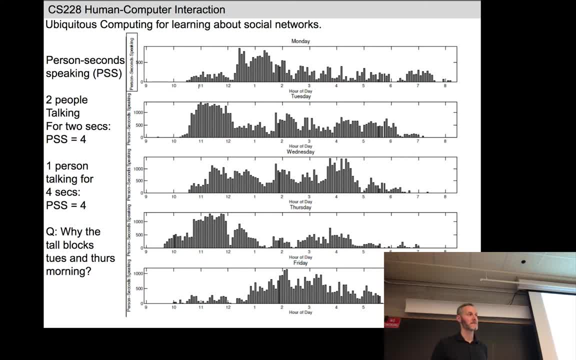 if they're apart. Um, well, generally I'd say like they all seem to share a schedule, at least in some ways, with, like those matching blocks, or the Friday trends or the Monday trends. they, for some reason, they're all seem to be matching up in some way. 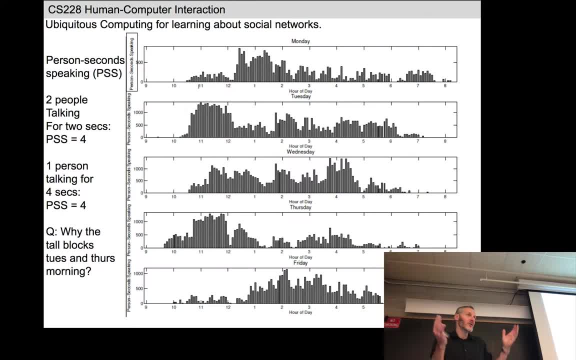 which, again from context, you'd you'd sort of imagine, right? So I said 24 graduate students. graduate students is a much smaller pool than the undergraduate pool, So they're probably taking similar courses and seminars and they're probably together Tuesday and Thursday morning. 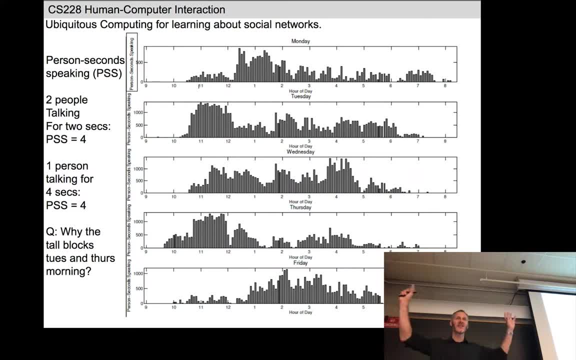 right, It would be unlikely that they're all in different places And it's just at this particular time that there's a lot of speech. Let's assume they are together Tuesday and Thursday morning. Are they in a lecture or are they in a seminar? 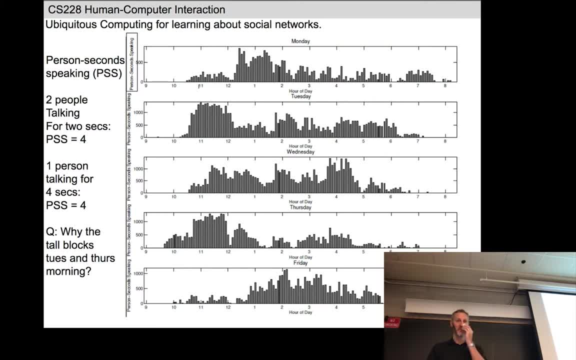 Seminar. Why a seminar? Absolutely So importantly, as I mentioned before, the microphone is very near their mouth and near their ears, So this device is able to distinguish between are they talking or are they listening to somebody else talking, And PSS is only measuring them talking. 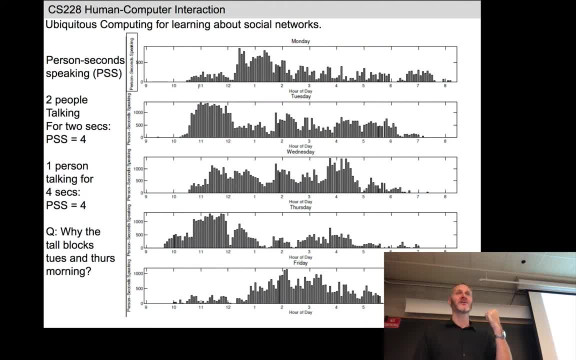 It throws away, for the moment, information about somebody else talking. So the 24 graduate students themselves are doing much more talking Tuesday and Thursday morning than they are as a group on average the rest of the working week. right, So we're we're already starting to infer something about this. 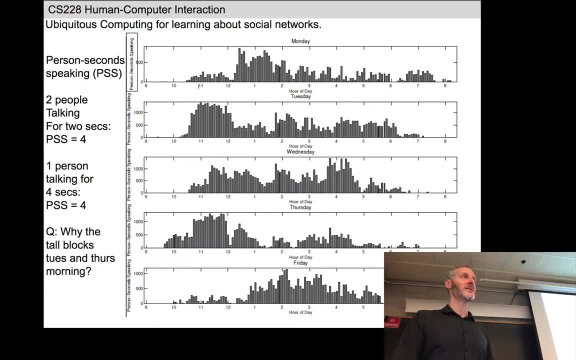 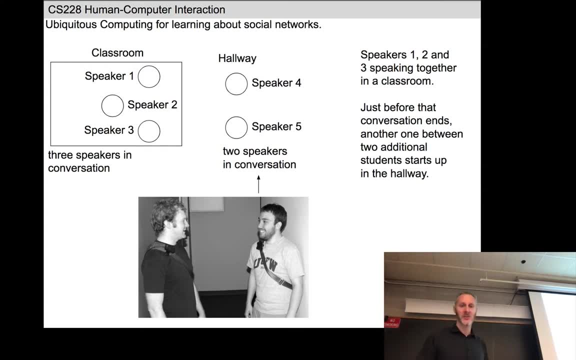 this group, not necessarily about social dynamics, yet. Okay. so let's have a look now at starting to zero in on social interaction. Let's imagine an example here. So, at a particular point in time, imagine we have three of the speakers that are in a classroom or they're together somewhere. 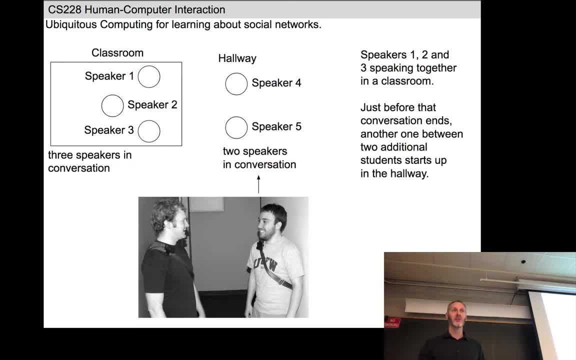 They're in a coffee shop and the three of them are involved in a conversation Outside that room. in a neighboring hallway. speakers four and five are also in conversation. Imagine further that the conversation inside the room- uh, just before it finishes, the conversation out in the hall starts up. 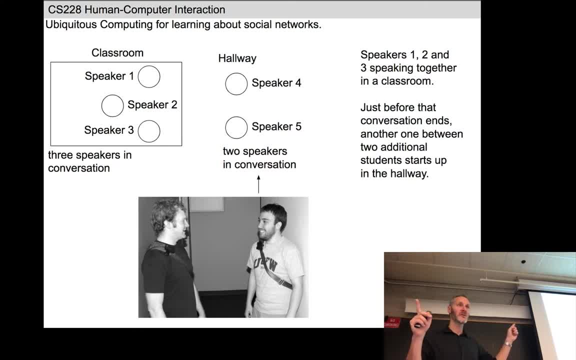 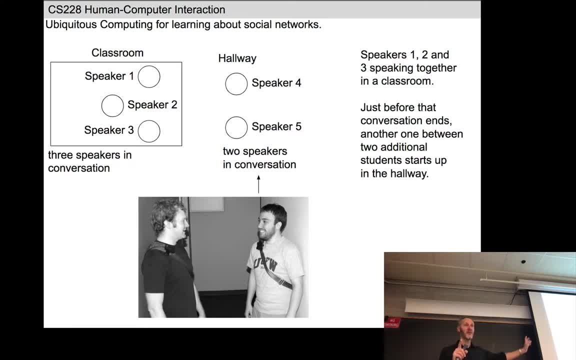 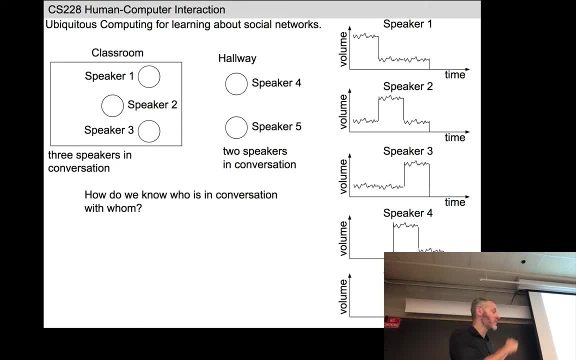 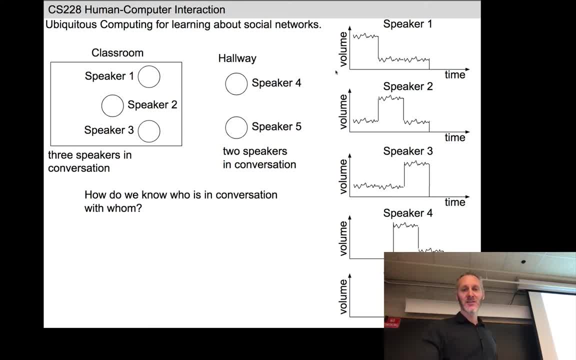 these five speakers, we might notice that for a certain period, for a certain period, Speaker one's volume is high and then their volume is medium. Same thing for Speaker two and Speaker three, And we might notice that this non zero volume or medium and high volume covers the same period of time. it suddenly grows silent, for 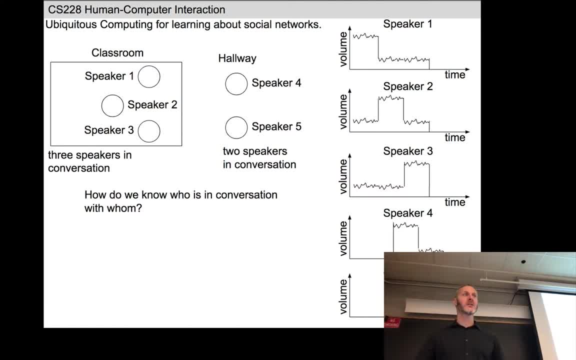 all three, or at least there's no more speaking they go into. they go into a quiet study session or something else happens and the conversation ends. same thing for speaker four and five. how would we take this raw data and discover that, in fact, the first three speakers were in conversation? 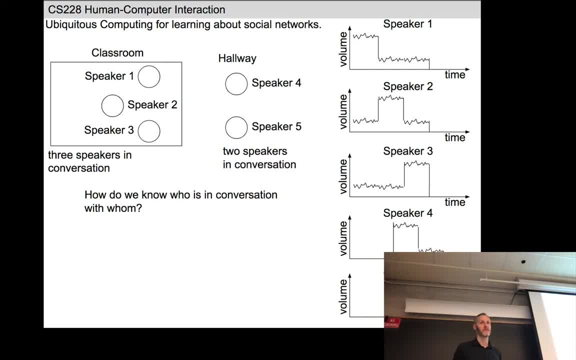 and then speakers four and five. well, if you could say that speakers three and four weren't in conversation because they're speaking, speakers three and four possibly they're. they're definitely speaking at the same time. there are conversations where people are speaking at the same time. it's a good start. 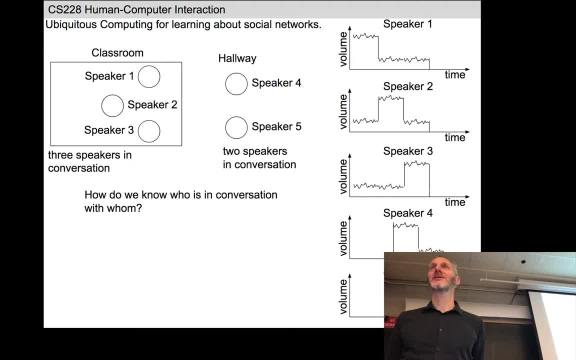 they match up right. so i arranged these five plots vertically as a hint. right, we're looking for temporal coincidence: things are occurring at the same time. right, we might have people that are actually speaking at the same time but are still doing it as part of a conversation face to face with one another. so how do we look for this? 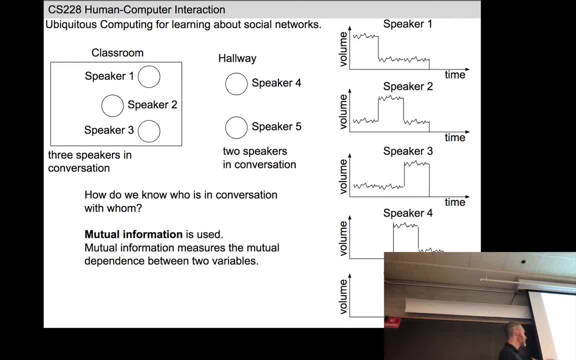 temporal coincidence. we're going to use- or the investigators use- something known as mutual information. we're not going to go into the mathematical foundations of mutual information. for our purposes it's like correlation: it tells us about the mutual dependence between two variables. so let's apply this idea of mutual information. let's start to march from left to right along. 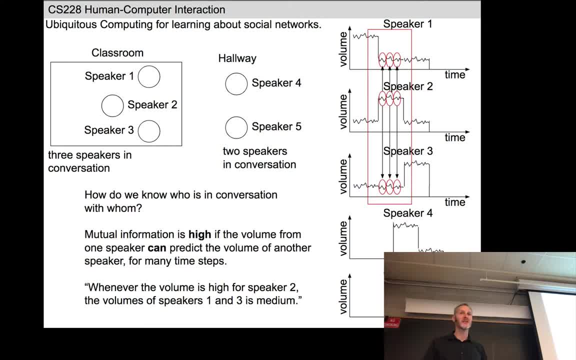 these five panels and at each point in time we're going to pick one of the five panels and take the amount of volume and compare it against the amount of volume in the other four panels, among the other four speakers, and we might notice, for example, that there is high mutual information, actually just during this period. 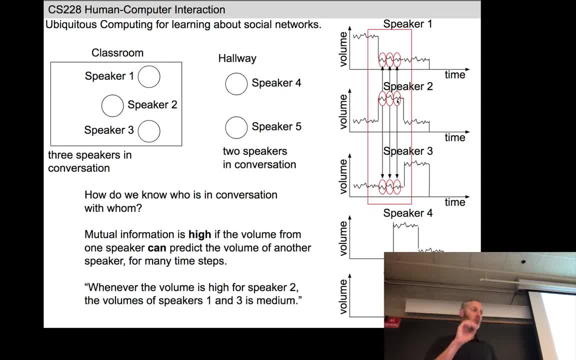 here during this period. whenever speaker two's volume is high, the speakers for the other two volumes register medium volume for that period. so another way to think about mutual information is whenever i measure one thing, in this case high volume for speaker two, i can be confident if there's high volume here. 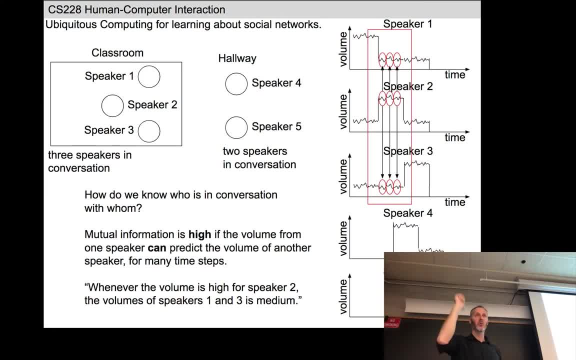 i can predict medium volume for speaker one and speaker three, and at least within this time interval. i'm always right. that's mutual information. so there's high mutual information here. there's also high mutual information during this time period. i can be confident that whenever speaker three's 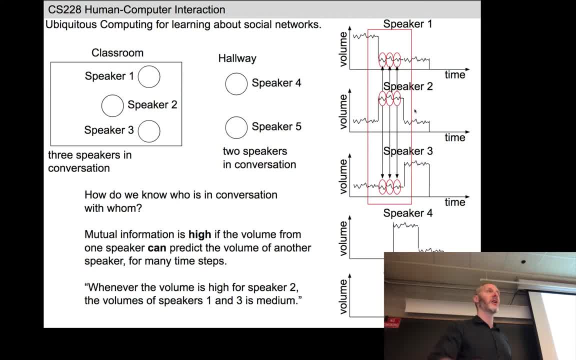 volume is high volume and speaker 2's volume is medium. So among these three speakers as they march from left to right during just this period, there is high mutual information. The particular correlation between whose volume is high and whose is medium changes but mutual information is high If we look at this time period. 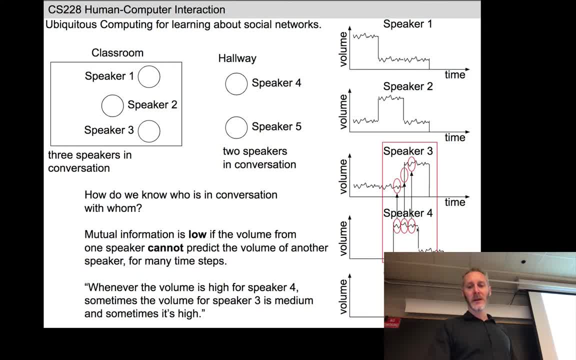 here and we look at speaker four. speaker four volume is always high but I cannot be confident that the high volume for speaker 4 predicts the volume of speaker 3.. There is low mutual information between speaker 4 and speaker 3 during this period. so you can imagine as I'm computing mutual information during this. 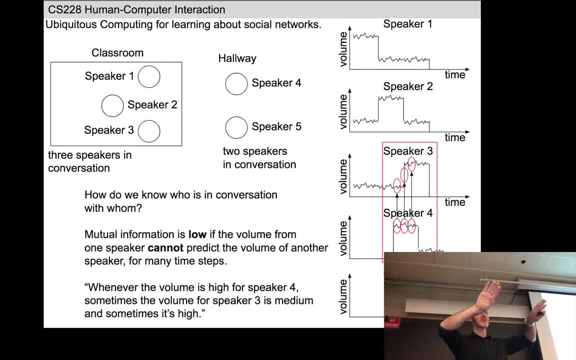 time period. the distance between speaker 3 and speaker 4, as theported parameters, can be calculated by S and then S. This gives C and C or L, the degree universities and I, so we will. Fermerde question when speaking is increasing, The more mutual information I detect between volume. 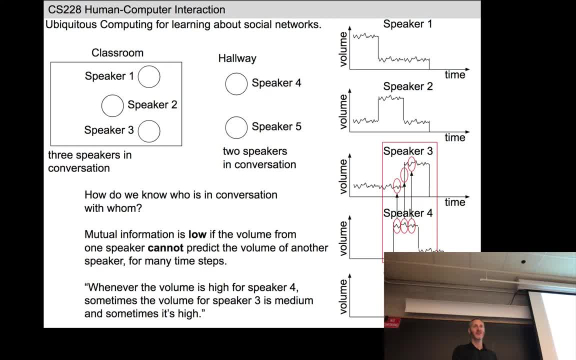 levels of different graduate students for the same slice of time, the more confident I can be that they're in a conversation, even if they're speaking over one another. So far, so good. Okay, so that's how we're starting to go: from raw volume information to social network inference. So if I take just these five, 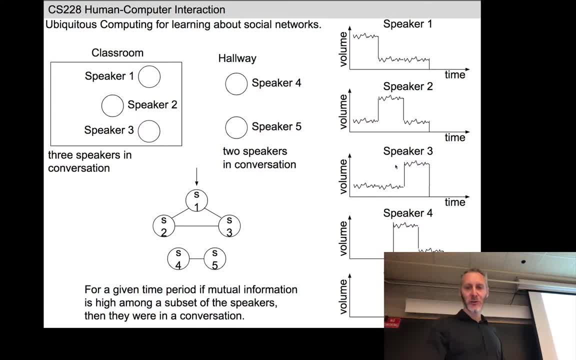 graduate students. I can be confident that, at least for this time period, these three speakers were in a conversation. So we're going to set some threshold and if mean of mutual information goes above that threshold, I predict these people were in a conversation And I'm going to. 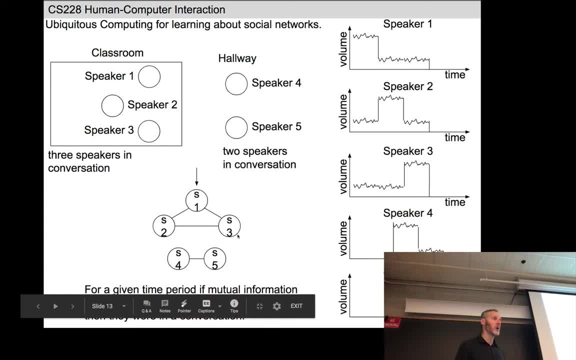 represent it using a social network. So in a social network we have nodes and edges. The nodes represent people and the edges represent some social relationship between them. In this case, in our purposes, an edge is going to represent that that pair of graduate students was. 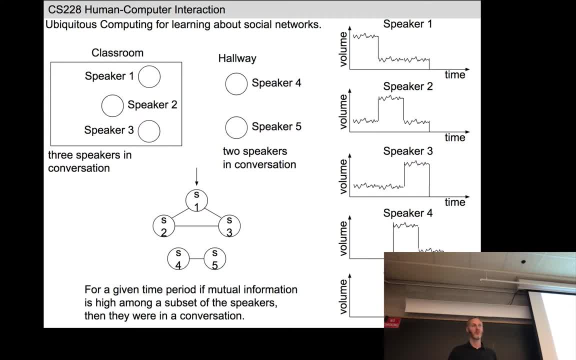 involved in a face-to-face conversation with each other for some period of time. We don't know whether they're friends. we don't know if they're competitors. we don't know if they're arguing with one another or agreeing, we don't know. 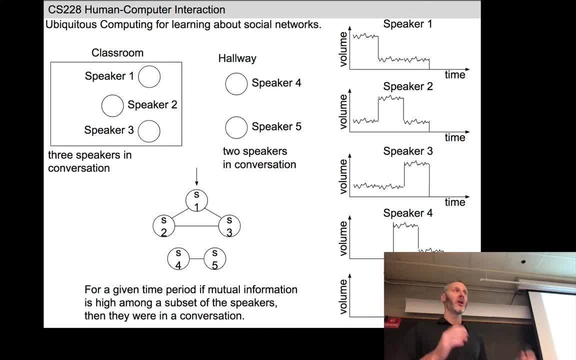 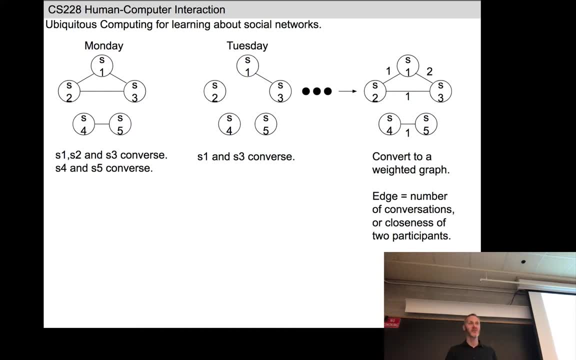 anything else, We only know they were together in the same place and they're involved in a conversation together. If we repeat this process over lots of these time slices throughout this six-month period, we can detect multiple conversations among different subsets of the graduate school students at different points in time. Every time we predict. 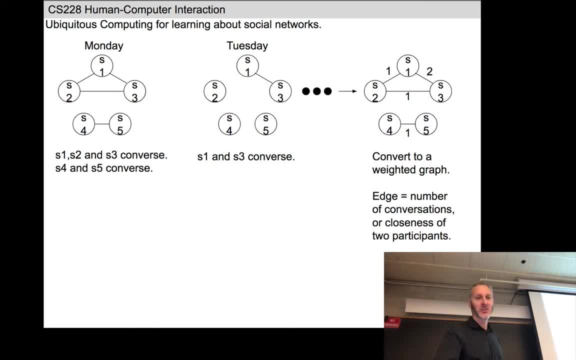 a conversation. we're going to add an edge to our network of twenty of them drinking four nodes. if we go to add an edge, like between s1 and s3, and there's already an edge there, then we assign a number to that edge, which is two. so we're going to now have a weighted social network. 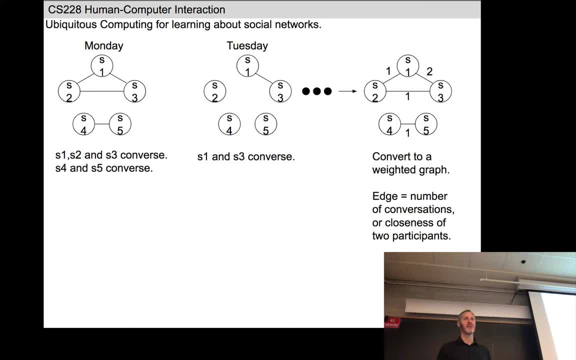 so the edges have weights, the weights are integers and the integers represent the number of distinct conversations that that pair of graduate students were involved in face to face. okay, so now we've gone from raw volume information to a final network, which is our prediction about a particular kind of social dynamic. how often were they involved? 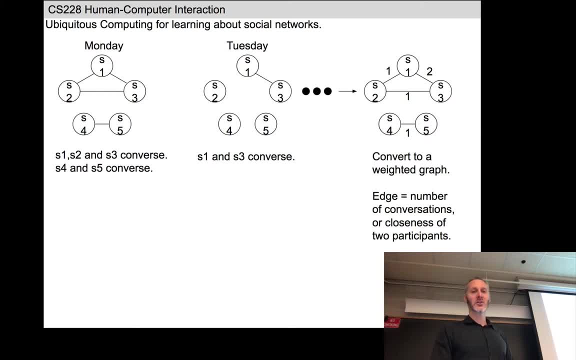 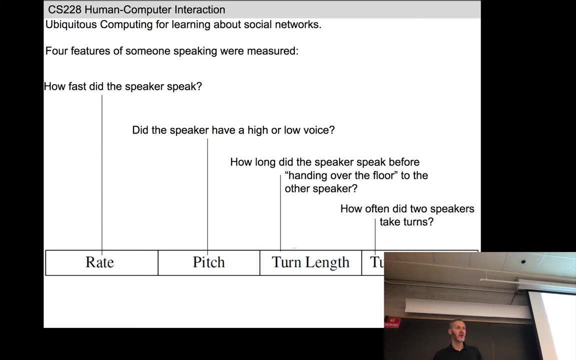 in conversation with one another. okay, that social network inference, that's step one. now that we do that, can we start to ask questions about social dynamics that would have been difficult or impossible to do before. what we're going to look at now is we're going to look at now, not just, not just. we used volume to infer the social network. 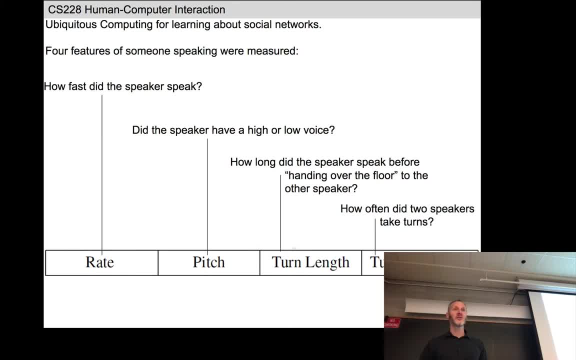 we're now going to use four other features of prosody, four other ways in which they spoke, but not what they said, and we're going to see whether their position in this social network that we just constructed, if that correlates with the way that they speak to other members of the group. we're 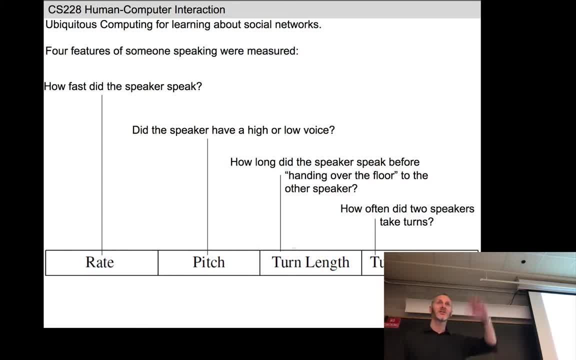 going to look at rate. how quickly did they speak? pitch did they speak? how frequency, low frequency, turn length: how long did somebody speak before they seated the floor to somebody else and, within a given conversation, what was the turn frequency? how short were the intervals during which one members 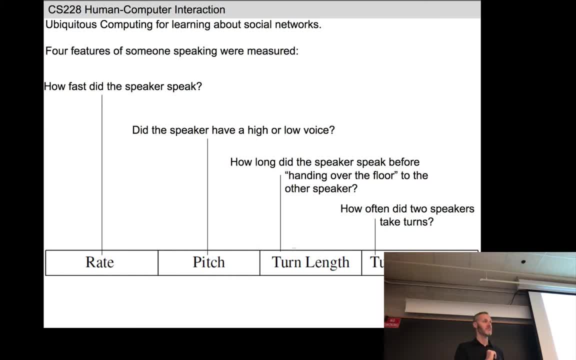 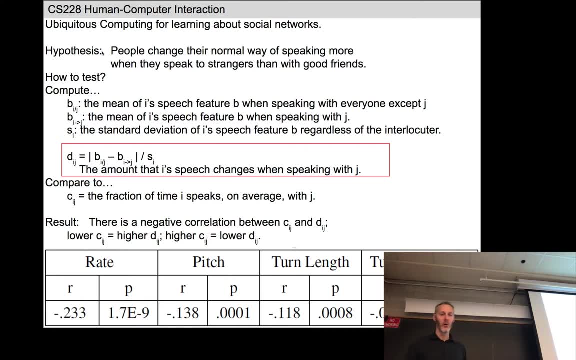 volume was high and the other volumes were medium. okay, so let's start with the hypothesis people change their normal way of speaking more when they speak to strangers than with good friends. okay, so there's several nouns in this sentence that we're going to have to pin down using metrics or data. so what do we? 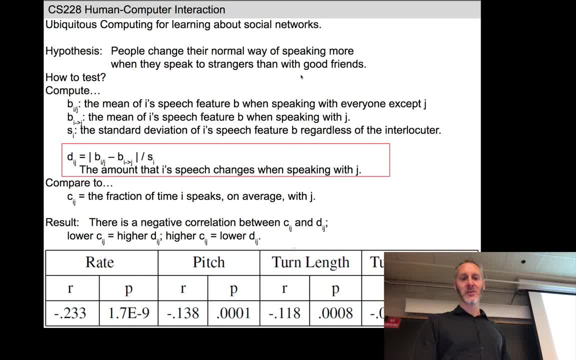 mean by their normal way of speaking? and what do we mean by strangers and good friends? let's start to test this hypothesis by computing B- I slash J, what that mean. B is going to represent one of these four features of prosody and we're going to ask about I, the person that's speaking. so, among these, 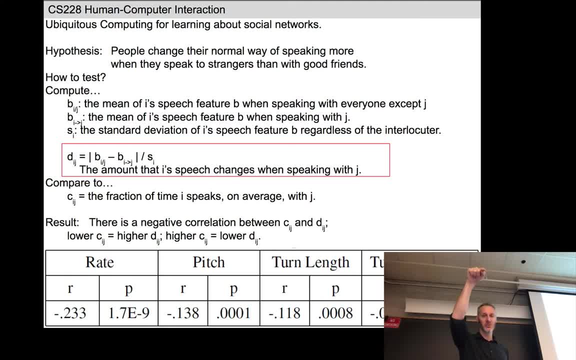 24 graduate students. we can pick one at random. that's graduate student I. when we can then look at this speech frequency, this speech feature such as rate: how fast did I speak? how fast did I speak when they were speaking to everyone else in the social network? all the other 22 graduate students? how fast they speak? 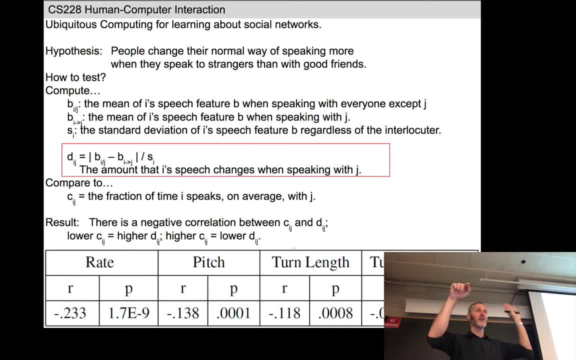 to sorry, just take the mean of that rate. so how quickly did they speak to the other 22 graduate students? then we can ask for the same graduate student, I? how fast did they speak when they spoke to J, the 24th graduate student? so how did? 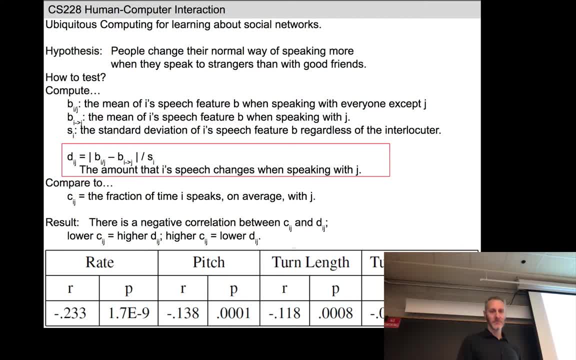 they speak to a whole bunch of other people in the group and J. we can then also compute S sub I, which is the standard deviation of the speech feature. so for a given graduate student, I, if they have high standard deviation, sometimes they speak slowly, sometimes they speak quickly if another graduate 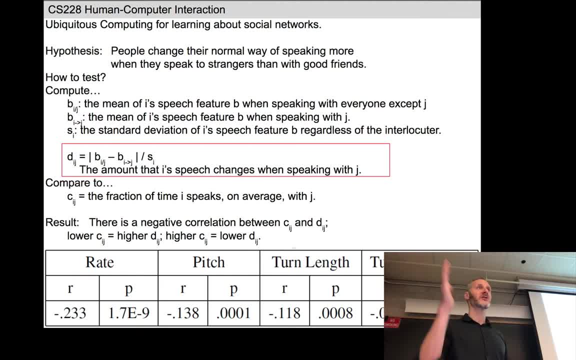 student I has low standard deviation. they tend to always speak at the same speed. humans differ in lots of different ways. we all have different ways in which we change how we speak. okay, we're going to put these three variables together to compute D I J, and D I J is going to represent the amount or how much eyes speech changes. 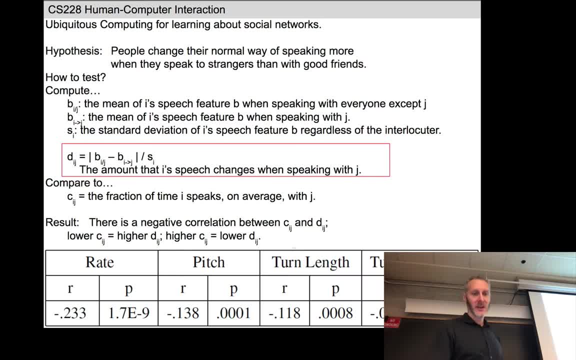 when speaking with J, right, so we're taking them their mean rate of speech. we're subtracting out their rate of speech when they talk to J. if they speak to J at the exact same speed as they talk to everybody else, these two B's will be equal. cancel each other out will be near zero and we're going to 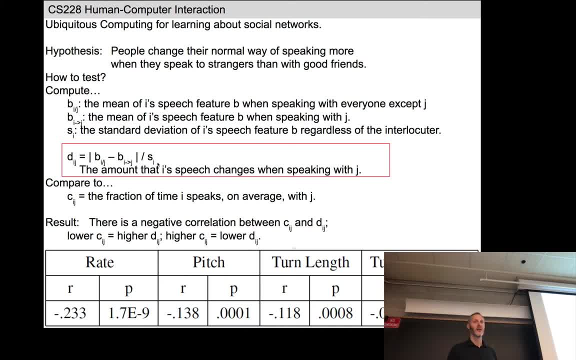 normalize. we're going to divide by standard deviation. we're going to try and ask how the rate of speech changes for all 24 graduate students. but some of those grad students their rate changes more compared to other graduate students and that part we're not interested in. it's a confounding variable. so we're 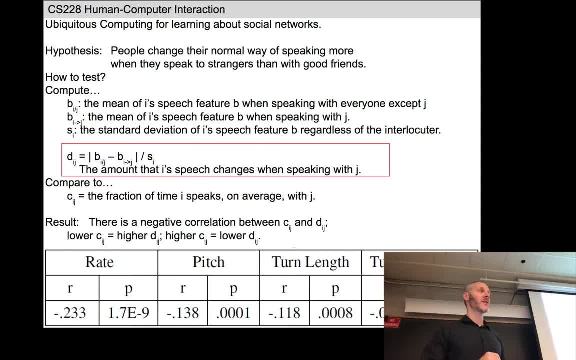 going to get rid of it by normalizing by S, sub i. so far so good. okay, so we know dij. if it's zero, that means i doesn't change the way they speak when speaking to j compared to everybody else. if dij is high is positive. the higher it is, the more they change their speech. 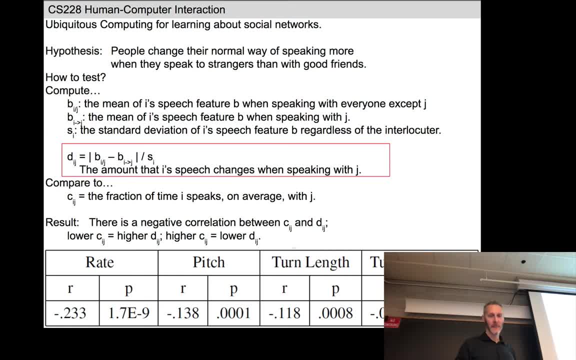 compared to j. okay, we're then going to compare d with c- the fraction of time that i speaks with j, okay. so now we've got c and d- the amount of time they talk to j and how they change their speaking behavior when speaking with j- and we can then go look for a correlation between c and d. 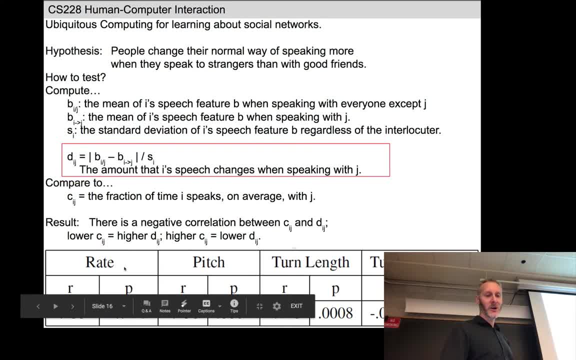 and it turns out that for all four, if we repeat this process, for all four of these features of prosody, there is a negative correlation. the higher c is the lower d is and vice versa. does that prove, does that provide support for the hypothesis or evidence against the hypothesis? 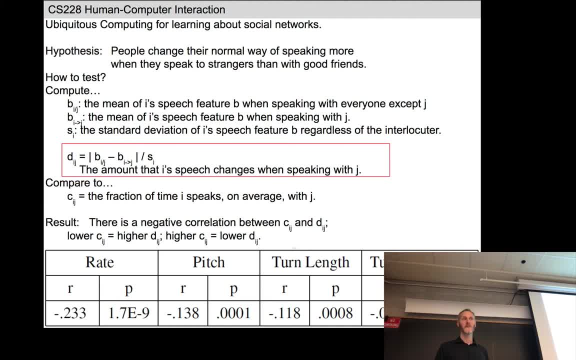 it proves it right. how, so? how does c and d relate to this hypothesis? uh well, I guess you you have to make the assumption that the longer you speak this someone, better they're not. that's right. so good friends is a bit of a subjective term here, right, we should. 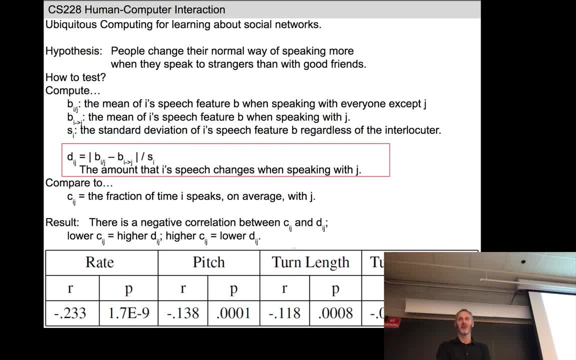 really replace good friends with people they often speak with during this six month period. yeah, but sort of correlation that even if it's negative, it's still a correlation that says: oh yeah, you're the way you speak to. somebody changes when you're more than they are. 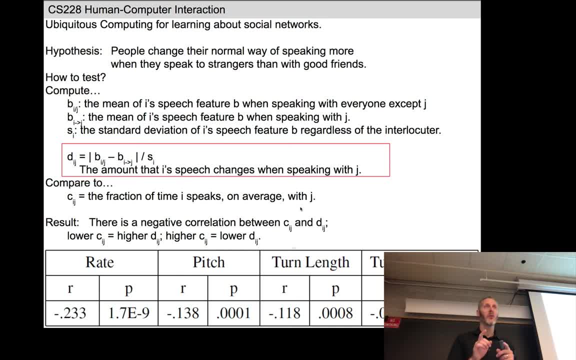 Exactly right. So let's take that example: The more you speak with someone, that means C-I-J is higher, You speak with them a lot, And D is lower. We're looking at. there's a detected anti-correlation here. 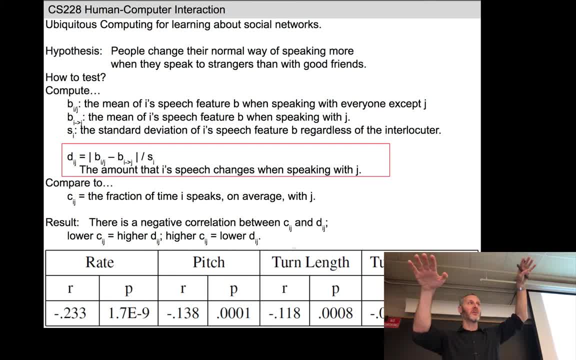 High C, low D. I know someone very well, I talk to them a lot And my D is low. The way I speak to them is the way I usually speak to other people in the group And maybe, more tellingly, is the opposite. 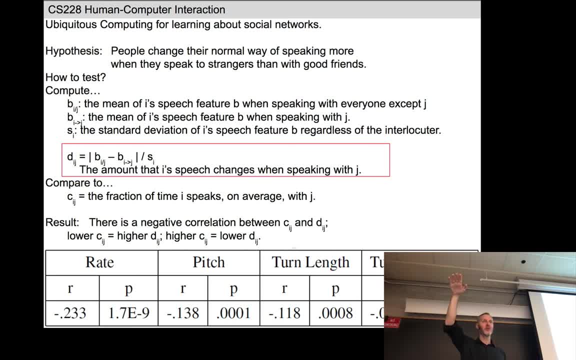 When C is low, I'm speaking to one of the other 23 graduate students that I rarely speak to during this six-month period. C is low, D is high. However, I normally speak. I'm now speaking differently to that person than I do on average to the other people in the group. 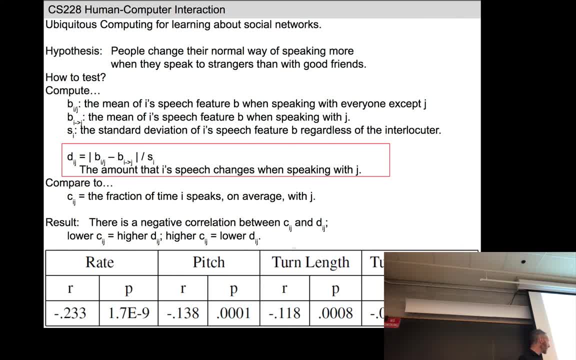 Okay, As I mentioned, this correlation is negative. There's an anti-correlation for all of these. So I change my rate of speech when I'm speaking to a stranger in the group, I change my pitch, I change turn length. It doesn't say whether I speak more or less. 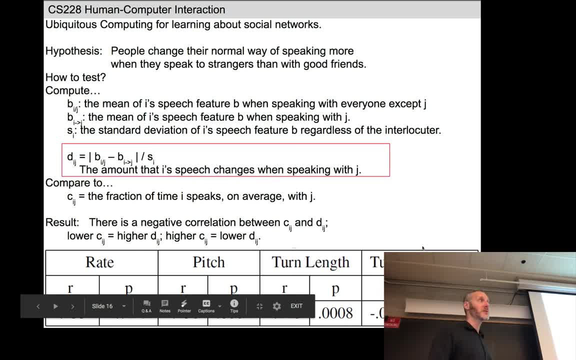 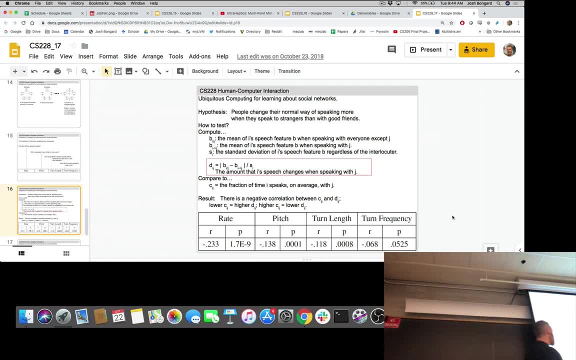 I just change my turn length. Same thing with turn frequency. We're going to end today by just talking briefly about P. P is, in statistics, a probability that our result is false, the null hypothesis. So maybe we're wrong. Maybe when C goes up. 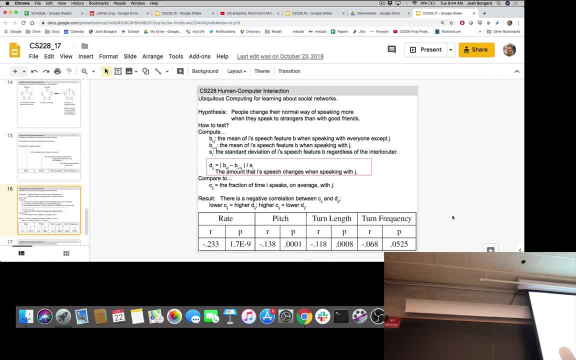 we're going to have a D. Actually it doesn't go down. The probability that I'm wrong if C and D relate to rate is extremely low. It's near zero. So I can be pretty confident that rate changes when I speak to a stranger. 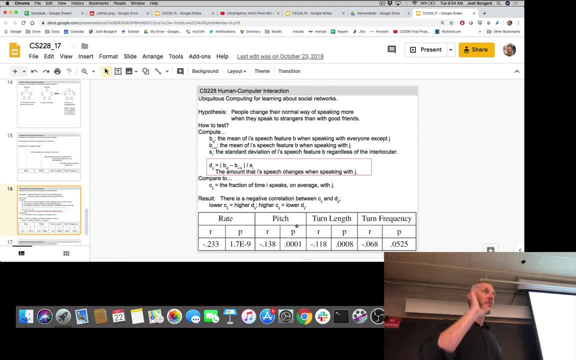 P is also low for pitch. I can be pretty sure that the pitch of my speech changes when I speak to a stranger. I can also be confident of it for turn length. P here is above 0.05, which for most statisticians.